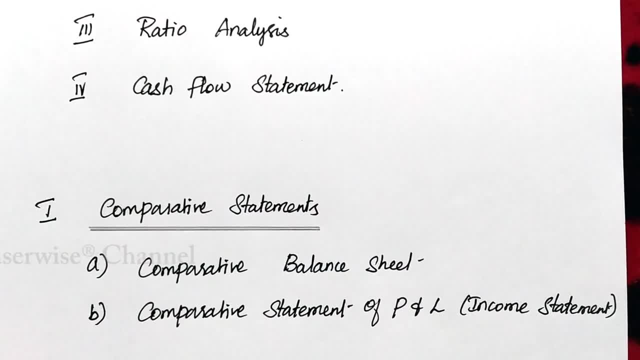 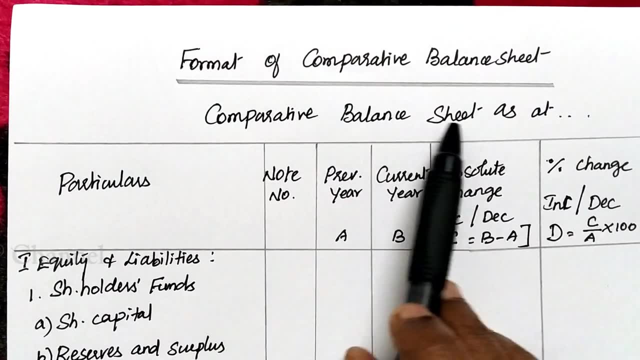 of comparative balance sheet, along with the financial statement analysis. Okay, the first two are comparative statements, The second one is comparative statement analysis. Then we will see the problem. Let us see what is comparative balance sheet, Let us try to understand the meaning of comparative balance sheet, along with the format. Okay, see the format Format. 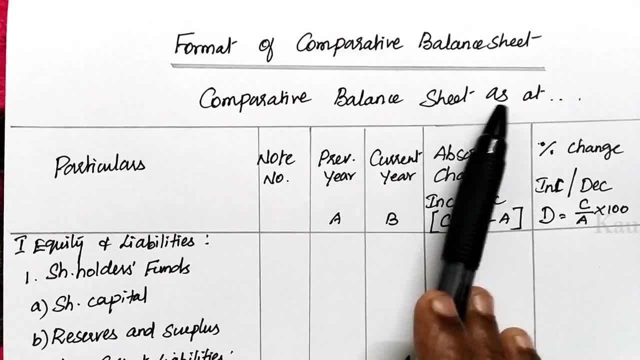 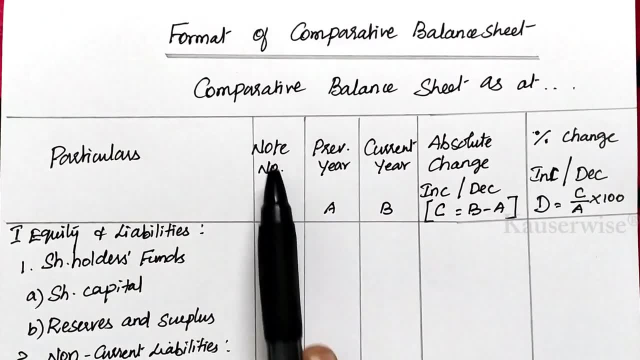 of comparative balance sheet. Okay, that is comparative balance sheet, as that two years will be given. Okay. so here we have different columns: The first one is particules, The next one note number, and then previous year data and current year data. First we need 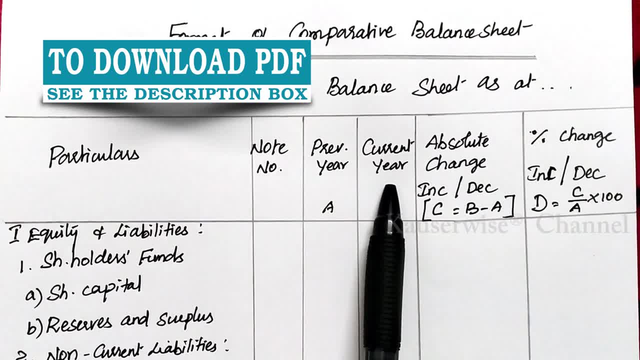 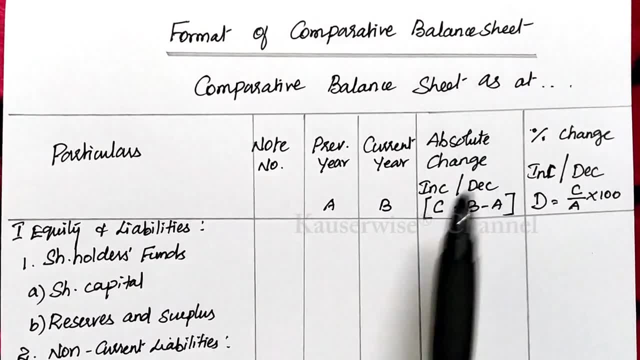 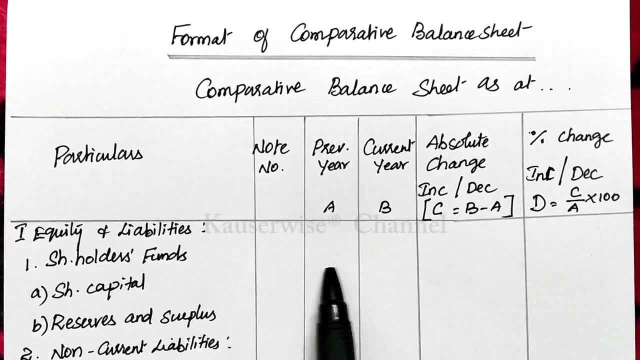 to enter year information, then only we need to enter the current year information, okay. and the next one is absolute change. okay, so absolute change means if there is any difference between previous year with the current year, that will be entered here. so when you find the absolute change, there is a. 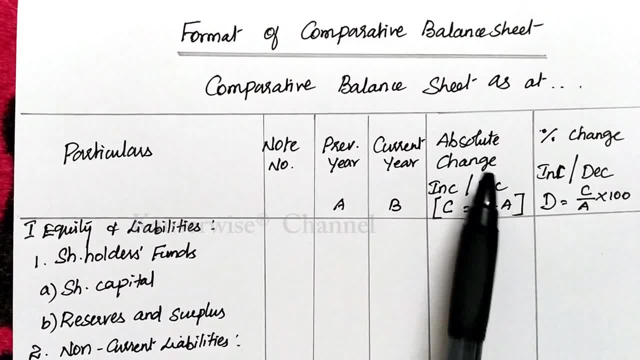 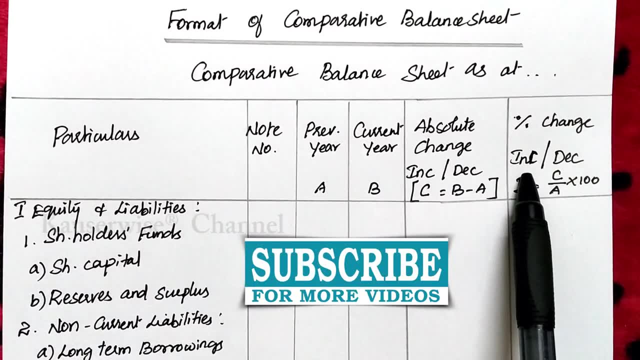 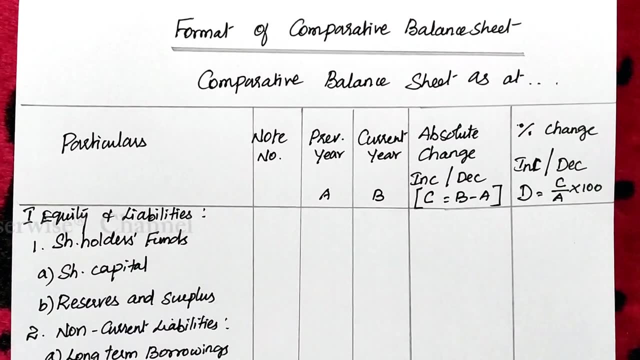 possibility of increase or decrease. okay, that is the absolute change. okay, that is a, c. and the next one is the last one is percentage change: of increase or decrease, whatever may be the result. that is absolute change. we need to find out the percentage, how much proportion the changes is okay. 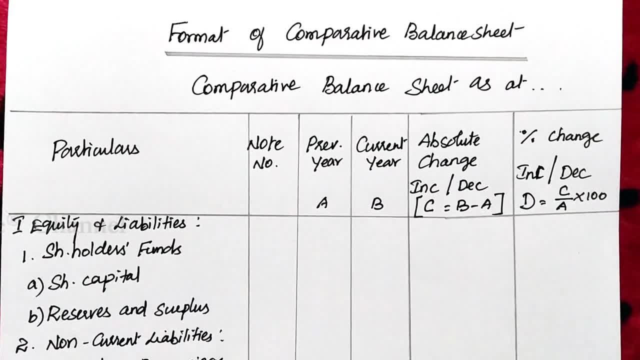 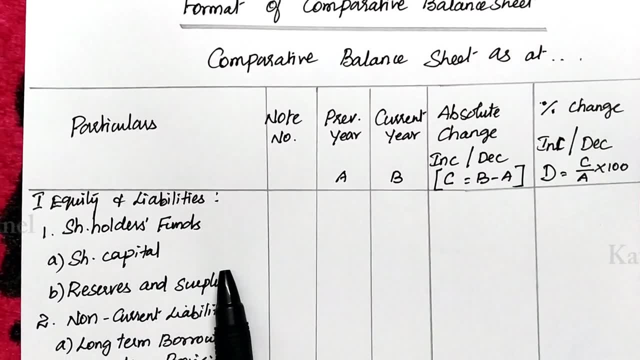 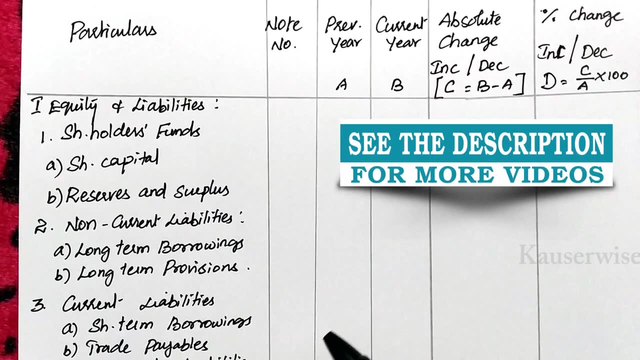 that will be calculated using this formula. okay, let us see one by one. the first one is under particulars. so this is the comparative balance sheet. no, the first part is equity and liabilities in equity. we know the format of preparing balance sheet according to the 🎞 circle box 🎞. 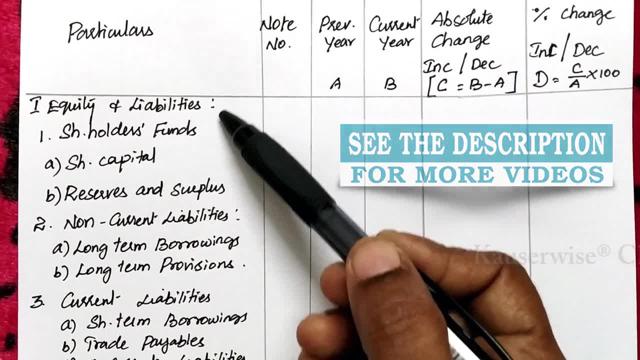 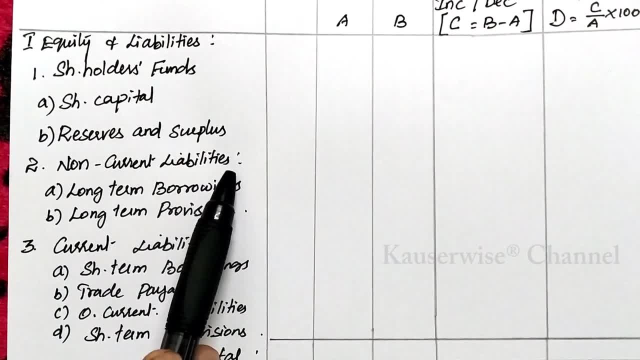 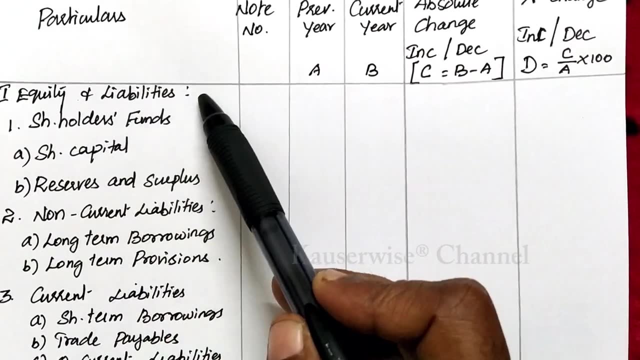 revised schedule. First, we need to enter equity and liabilities. under that, three components are there. First one, shareholders fund and the second one non-current liabilities. The third one is current liabilities. Okay, these are the three major components which comes under equity and liabilities, Okay, and the first one, shareholders fund. two components are there: share capital and 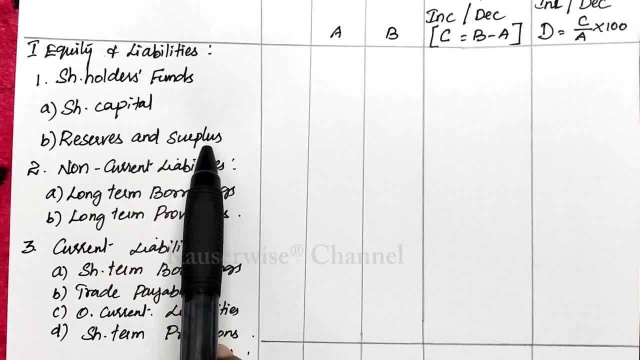 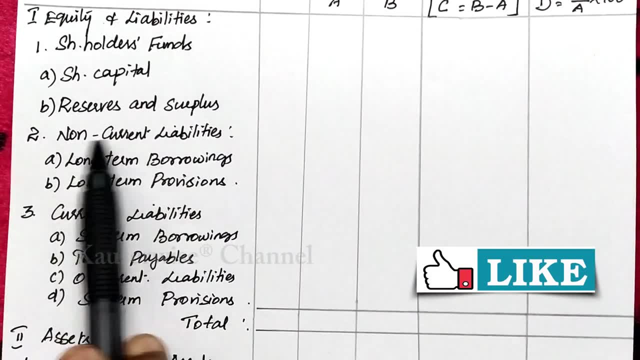 the second one, reserves and surplus- Okay, these are the two components which comes under equity shareholders fund. Okay, and the next one is non-current liabilities. Non-current liabilities are two things are there. One is long-term borrowings and long-term provisions, and the 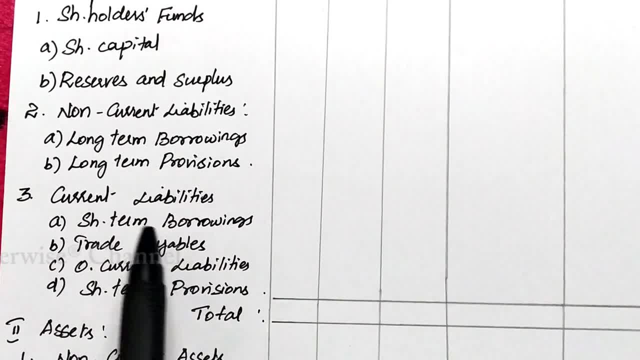 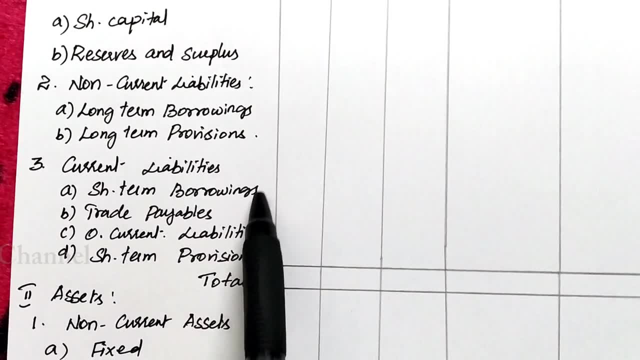 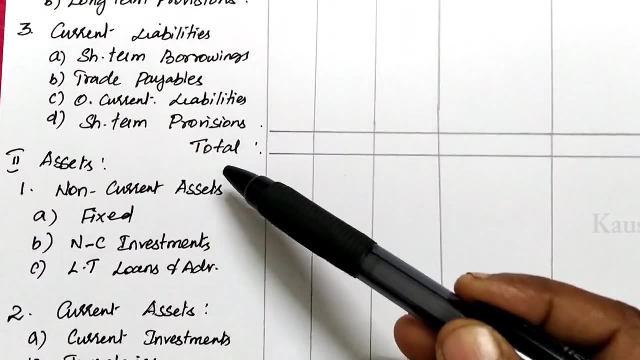 next one is current liabilities. So current liabilities are short-term borrowings, trade payables, other current liabilities and short-term provisions. So these are the various components which comes under current liabilities, Right? the second part is asset. Okay, under asset, there are two major components are there? The first one, non-current asset, another one is current asset. 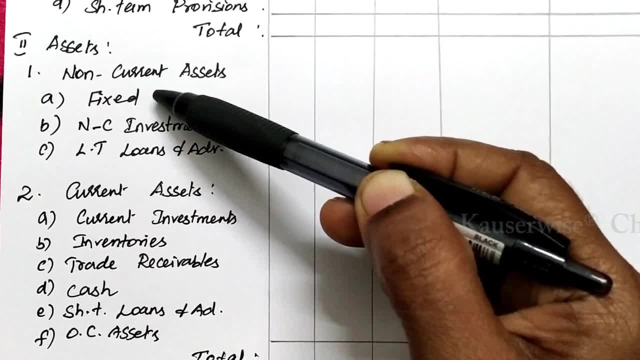 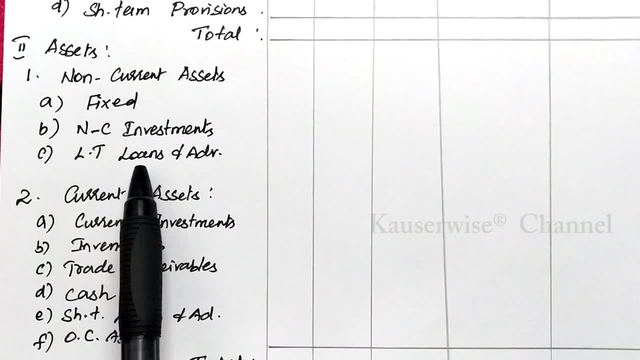 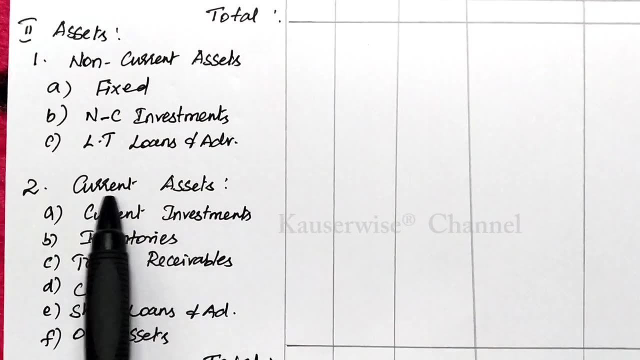 and a non-current asset. three elements are there. First, one fixed asset, the next one is non-current investments and the third one is long-term loans and advances. These are the three elements which comes under non-current assets. Okay, the next one is current asset. Under current 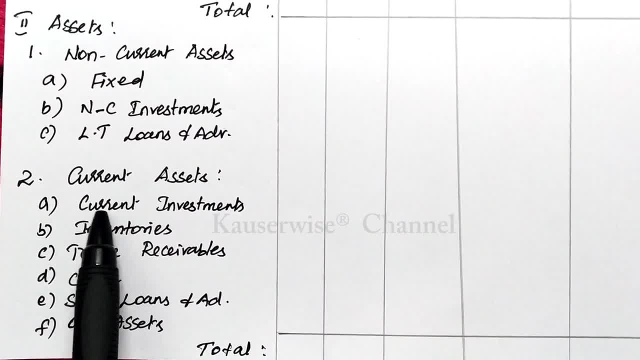 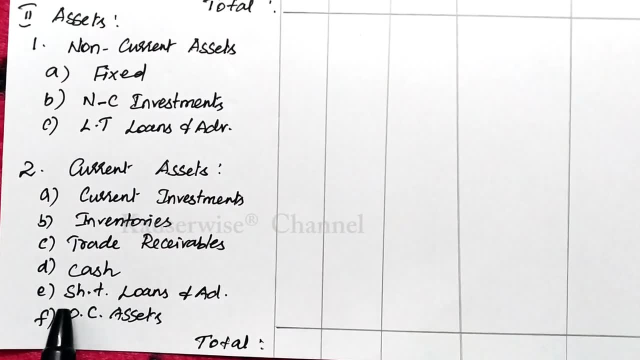 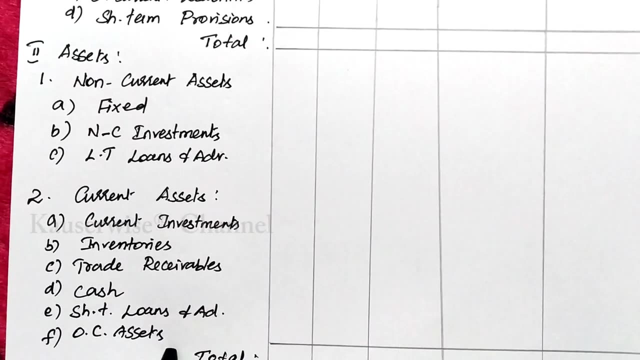 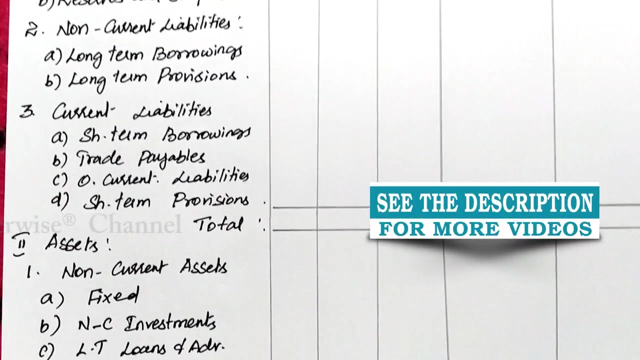 asset. these are the various elements: The first one, current investments, next one inventories, then trade receivables and then cash, and then short-term loans and advances. and the last one, other current assets. Okay, these are the various components which comes under current asset. Okay, this is the format of balance sheet according to the revised schedule 6.. Okay. 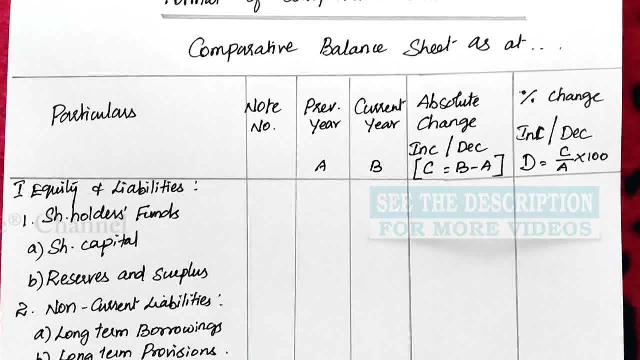 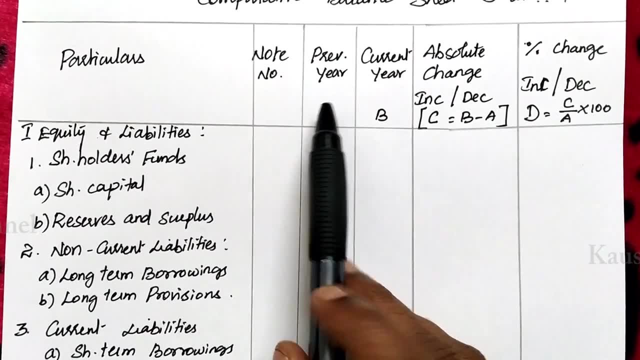 now. so with this we are going to see how to prepare comparative balance sheet. Okay, just enter all the elements of balance sheet item and then we need to prepare the balance sheet. So we need to write the previous year data and current year data. This information will be given. 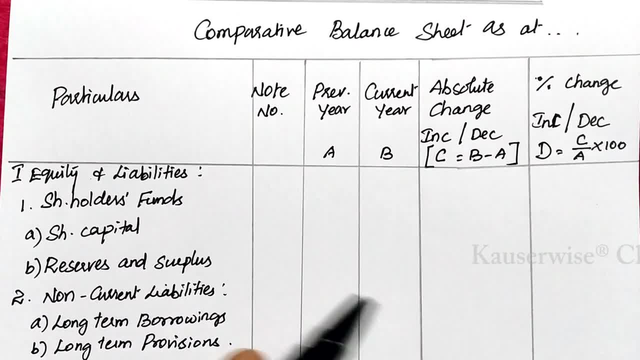 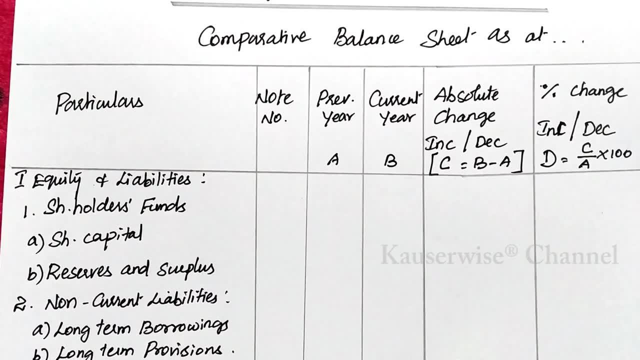 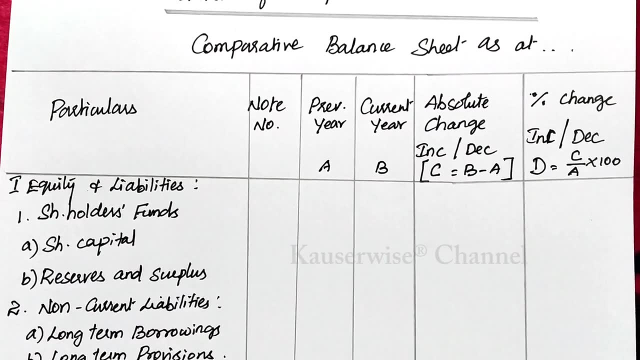 in the problem. So two years data will be. that is, two years balance sheet will be given in the problem. First we need to enter previous year information and then we need to enter current year information, For example, 2020 and 2019 informations are there In that case. first we 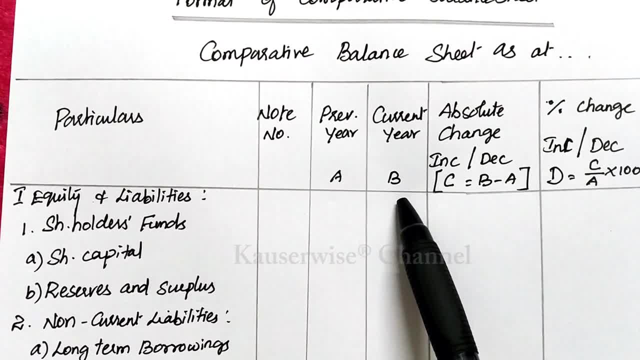 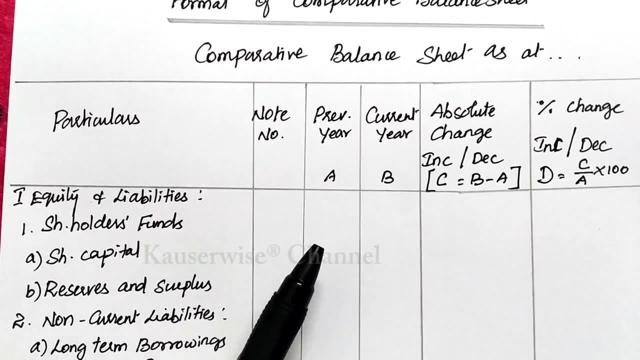 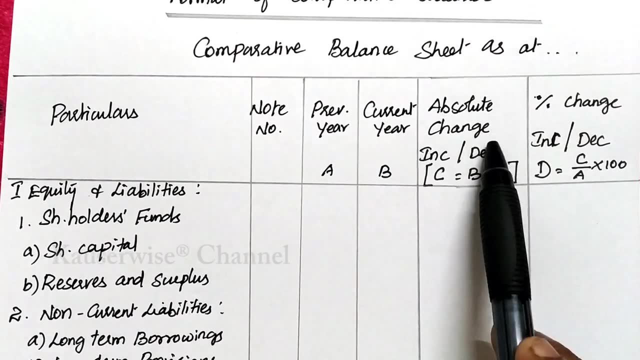 need to enter 2019 information, Then we need to enter 2020 information. So 20 is the current year, 19 is the previous year. Like that, you have to enter previous year first and then current year information. The next one is: we need to find absolute change, Absolute change. 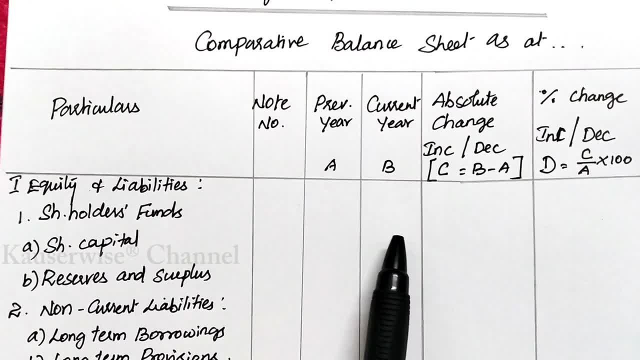 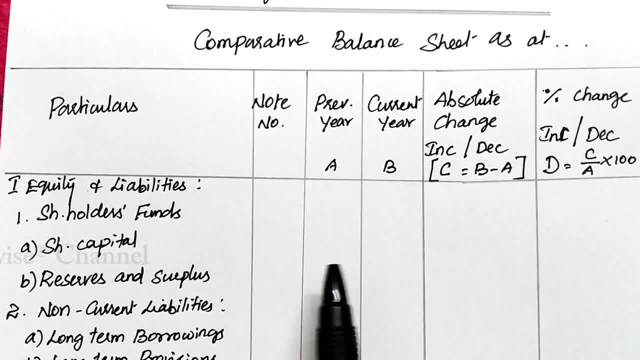 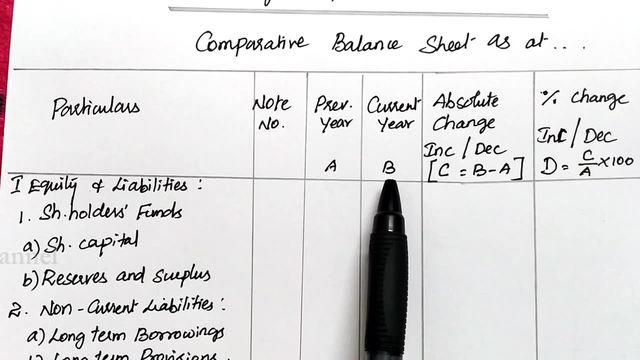 means we need to compare previous year with current year. Okay, when you compare two data, you can find some changes. It may be increase or decrease. Okay, that will be entered in this particular column. that is absolute change. Okay, so the first one is A, second one is A. 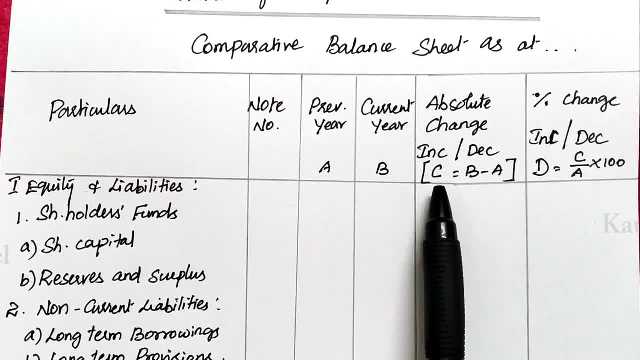 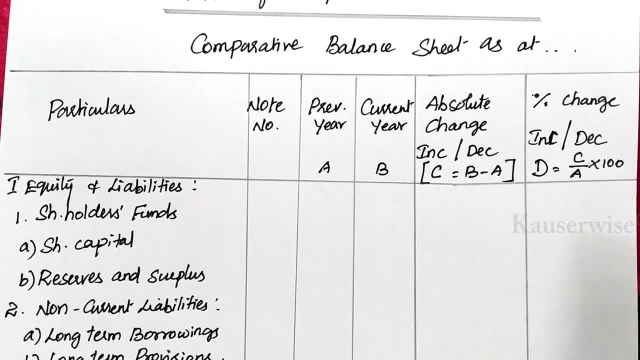 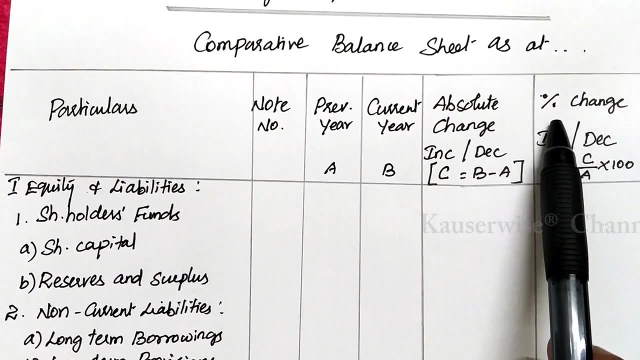 then we need to find C, C for absolute change. The formula is B minus A, that is, current year minus previous year. and finally, we need to find the percentage change. Whether increase or decrease doesn't matter. We need to find the proportion, that is percentage of change. Okay, the formula. 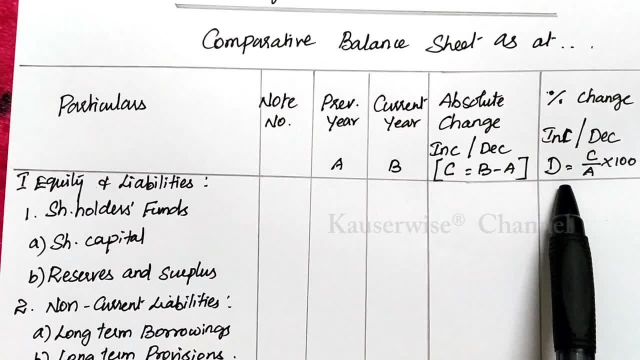 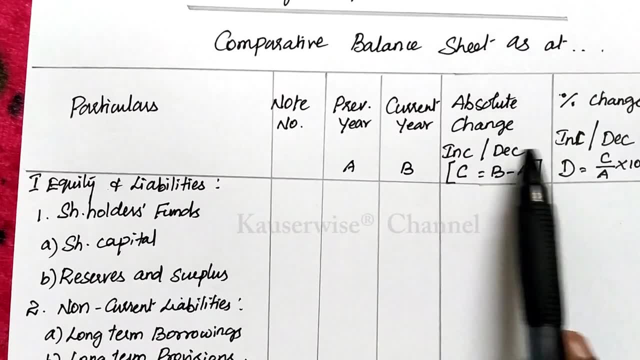 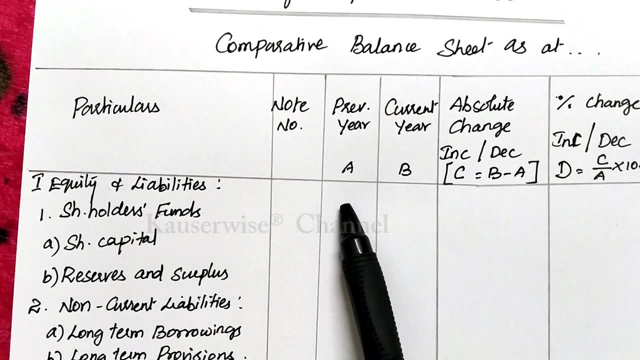 for percentage change is D. that is, D is equal to C divided by A into 100.. C for absolute change, that is, increase or decrease that will be taken into consideration divided by A. A means we need to take the base year. Base year will be previous year. The first information is the. 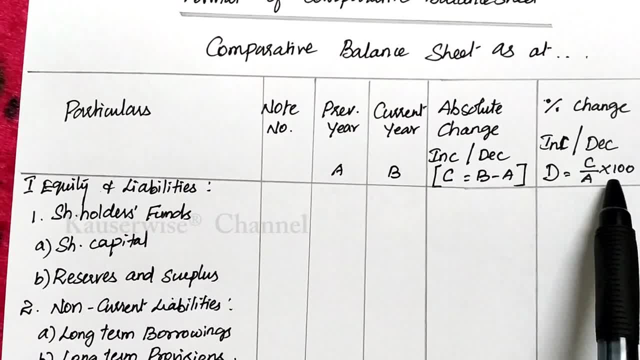 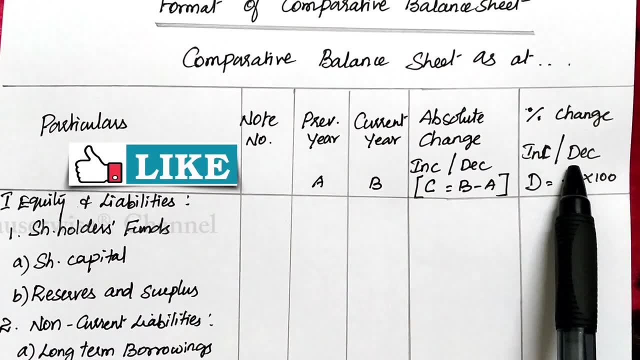 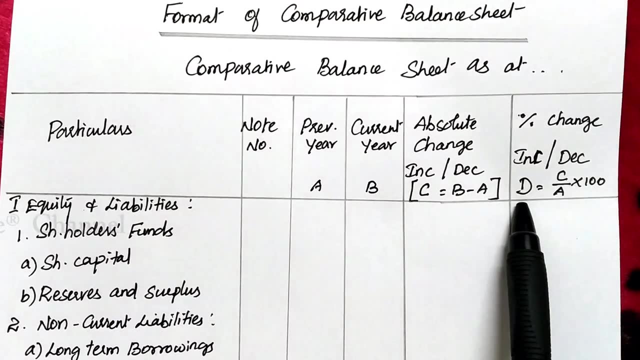 base year. Okay, with that you can find out the proportion into 100.. Okay, this is the formula to find out the percentage. Again, I repeat, C, that is absolute change divided by previous year data into 100.. So this is the formula to find out D. 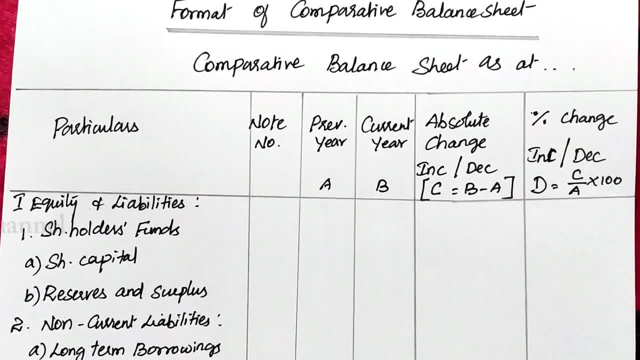 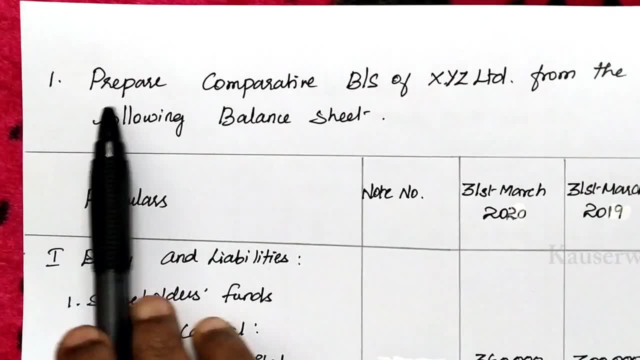 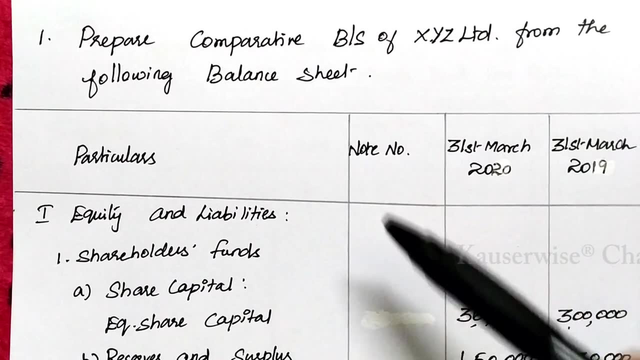 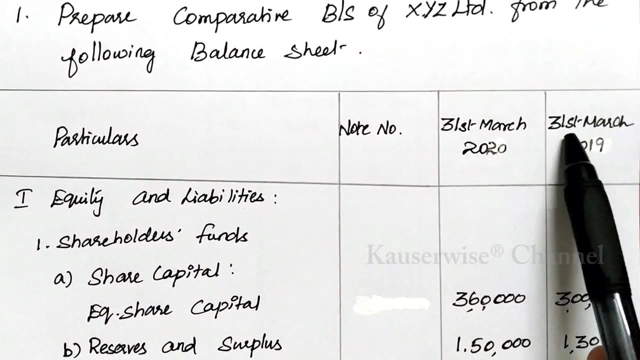 Okay, so this is the method to compare balance sheet between two different years. Okay, let us see the problem. See the problem: Prepare comparative balance sheet of XYZ limited from the following balance sheet: See here they have given some information. that is balance sheet for two different years. Okay, 31st March 2020 and 31st March 2019.. Okay, the first one is equity. 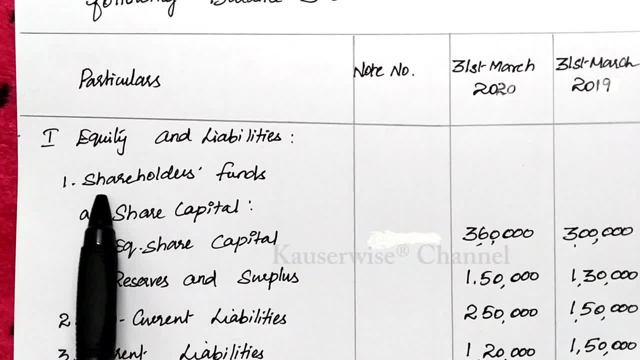 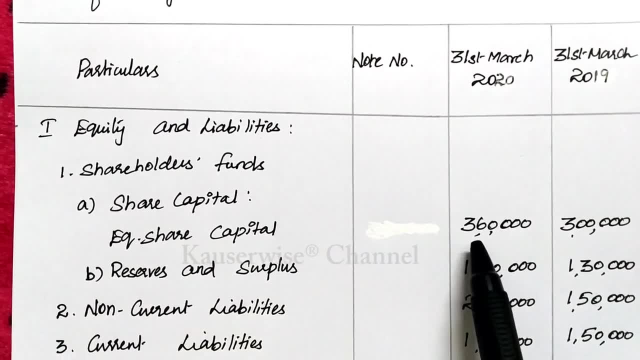 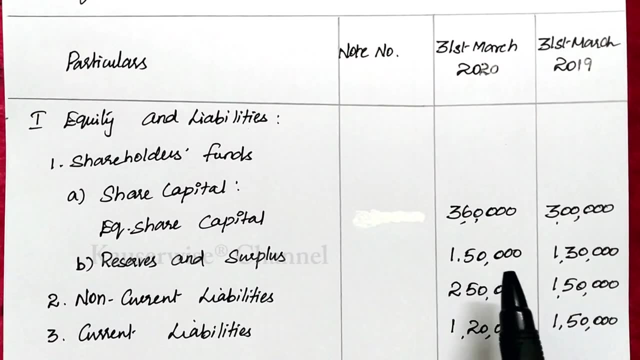 and liabilities Under that. the first component is shareholder's fund. Okay, under shareholder fund share capital. So here we have only equity share capital. How much? 3,60,000 in the year 2020 and previous year: 3,00,000.. Okay, and then reserves and surplus: current year: 1,50,000 and previous. 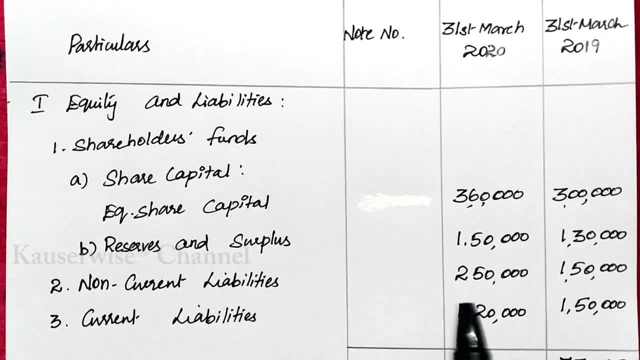 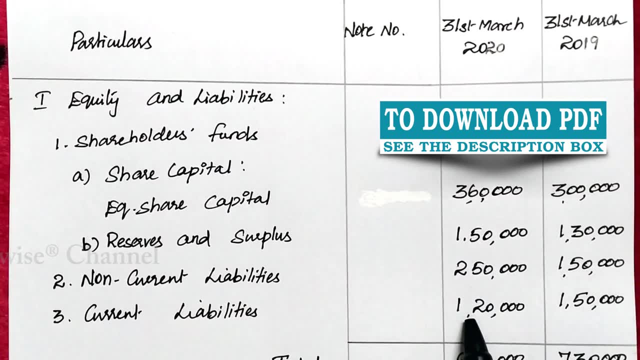 year 1,30,000 and then non-current liabilities: current year 2,50,000, previous year 1,50,000 and then current liabilities: Current year 1,20 and previous year 1,50.. So total current year liability is 8,80,000. 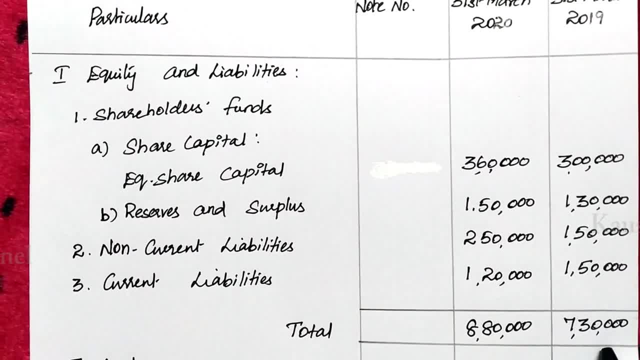 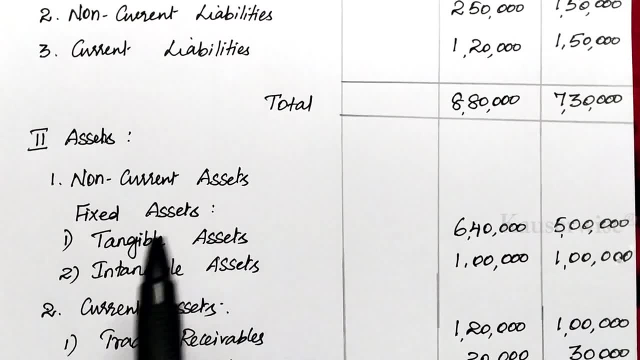 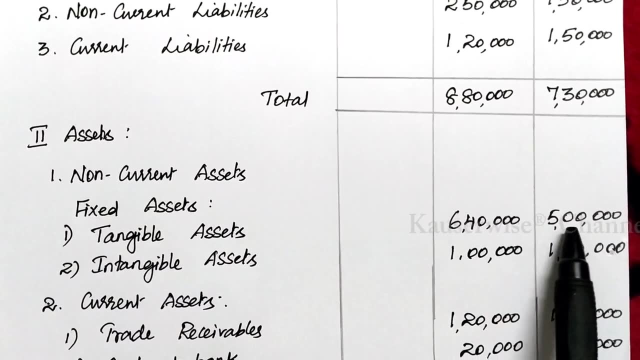 and previous year, total liability is 7,30,000.. Then second one is assets. So under assets, non-current assets or fixed asset, Under that tangible asset and intangible assets. Tangible assets for the current year: 6,40,000. previous year 5,00,000.. Okay, an intangible asset for the 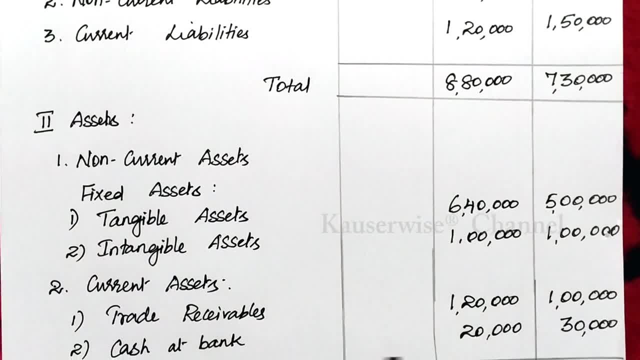 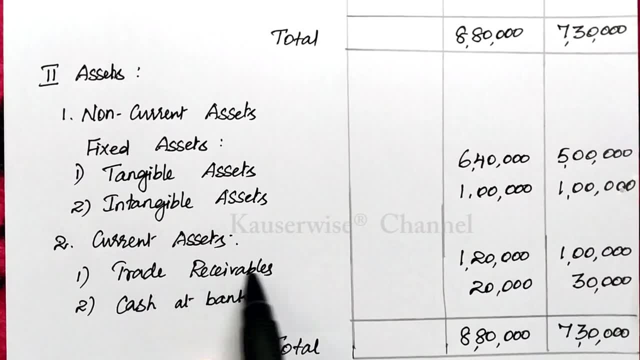 current year 1,00,000, previous year also. So under that, non-current assets or fixed assets also 1,00,000, and the next one is current assets. Under current asset, two components are there: trade receivables and cash at bank. So trade receivable for the current year: 1,20,000. 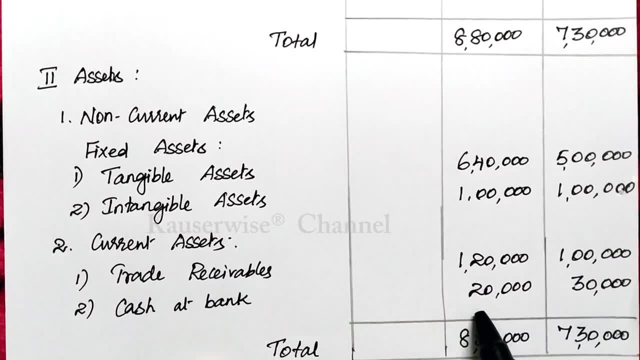 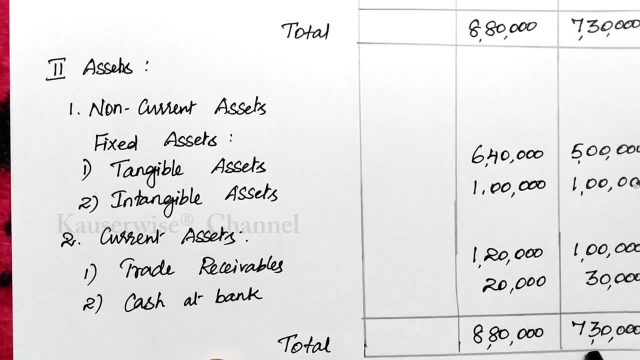 previous year 1,00,000, and then cash at bank: current year 20,000, previous year 30,000 and total asset for the current year 8,80,000 and total assets for the previous year 7,30,000.. 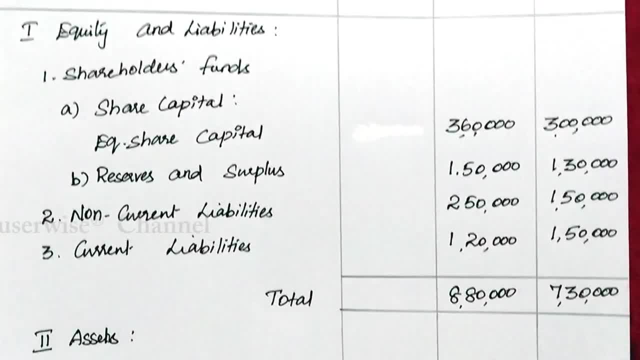 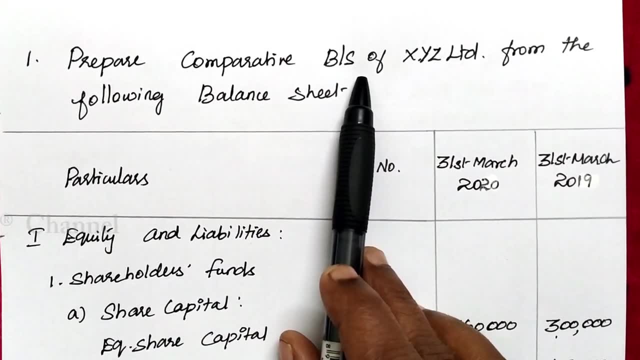 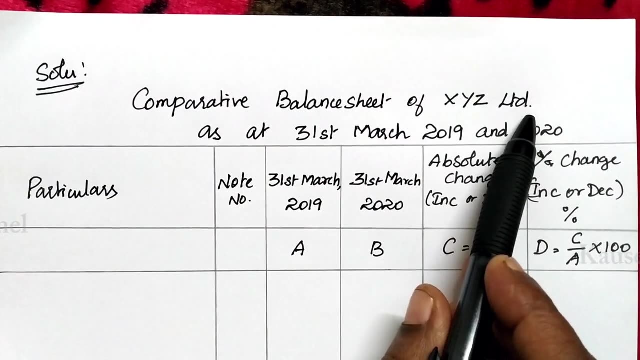 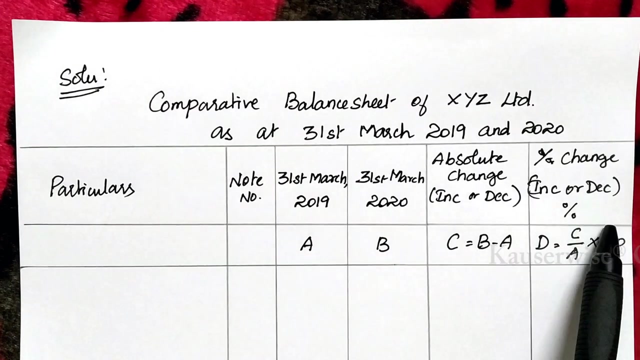 So this is the information given in this problem, that is, two different years balance sheet values are given. With this, we are going to prepare comparative balance sheet of the two different years. Let us see the solution. See the solution: comparative balance sheet of XYZ limited as at 31st March 2019 and 2020.. Okay, see, here we have different columns. The first one: 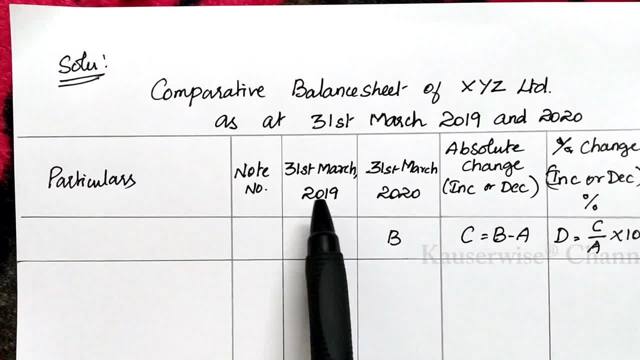 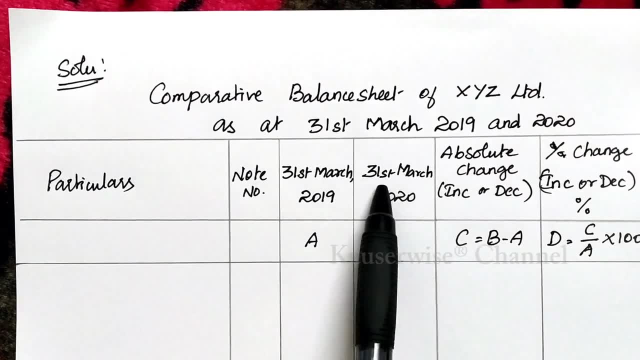 particulars and the next one note number, and then that is 31st March 2019, that is, previous year. A represent previous year Data and the next one 31st March 2020. that is end of current year. So B represent current year. 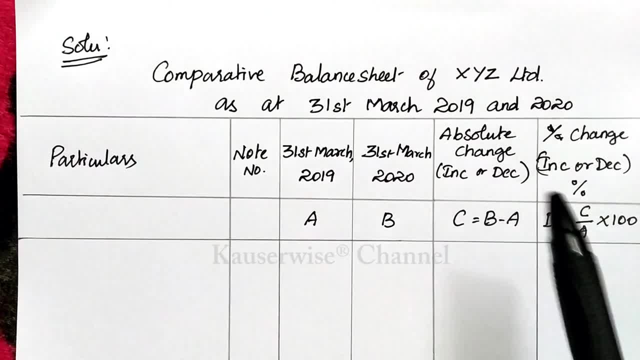 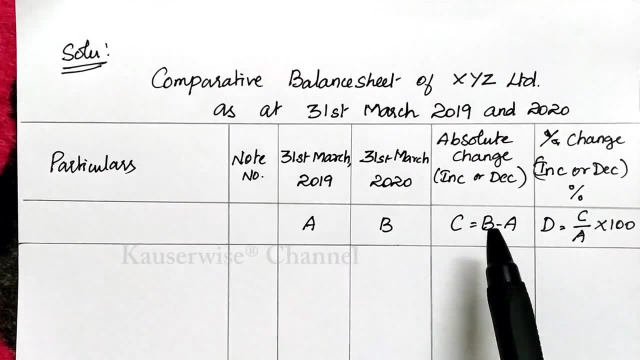 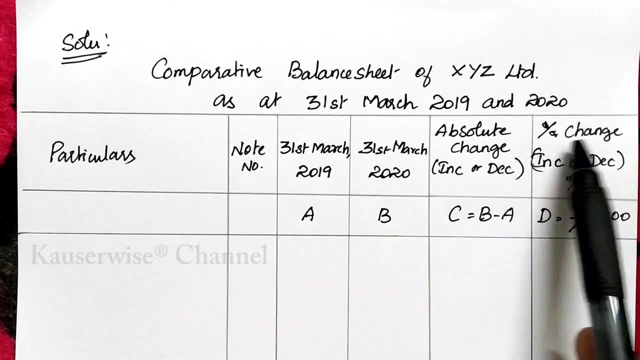 and then absolute change- increase or decrease. So we need to find out the absolute change by comparing current year with previous year. Okay, that is B minus A. You will be getting absolute change. that is increase or decrease, and the next one is percentage change. So after: 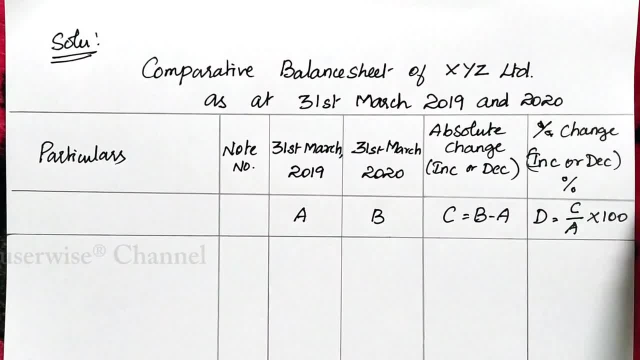 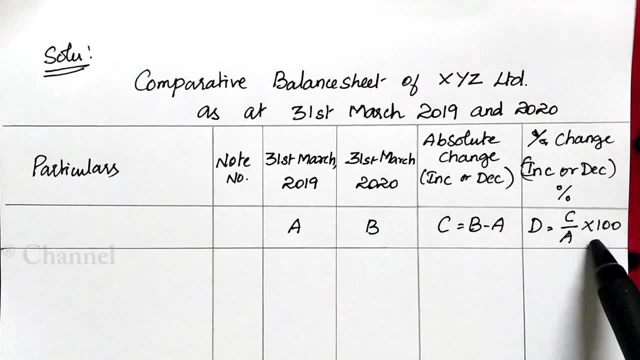 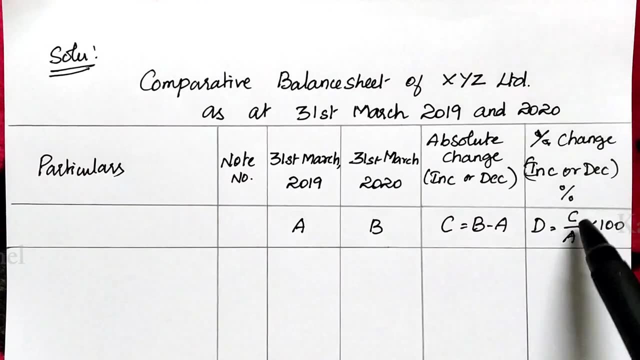 finding the absolute change. we need to apply the formula to find out the absolute change. That is: D represent percentage change. The formula is: C by A into 100.. C represent absolute change. that is increase or decrease. That is the absolute change divided by A. So A means previous year. 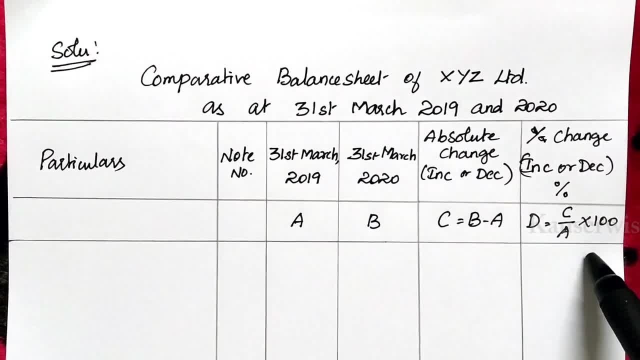 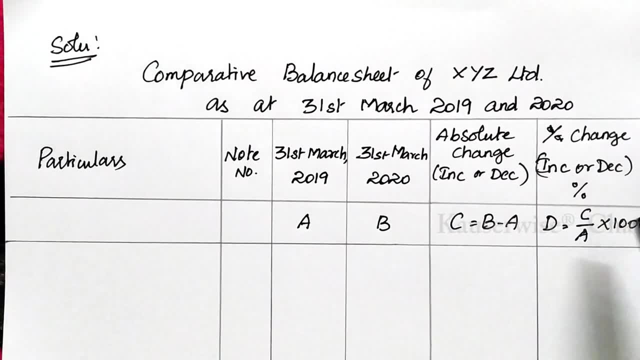 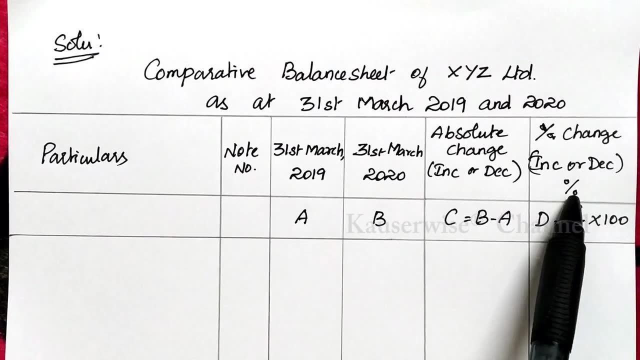 data. Okay, into 100.. So A is the base year to find out the percentage. We need to consider the previous year data to find out the percentage change. Okay, the absolute change divided by previous year data into 100.. Okay, this is the formula to find out the percentage change Okay. 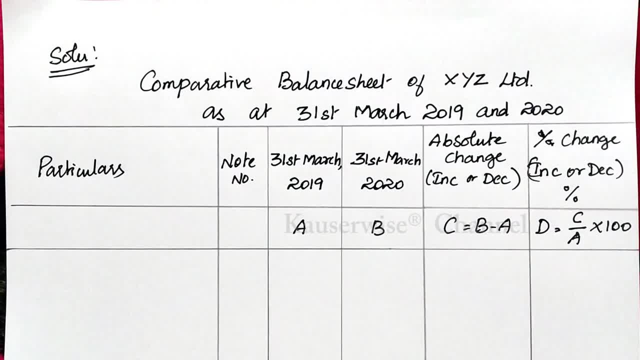 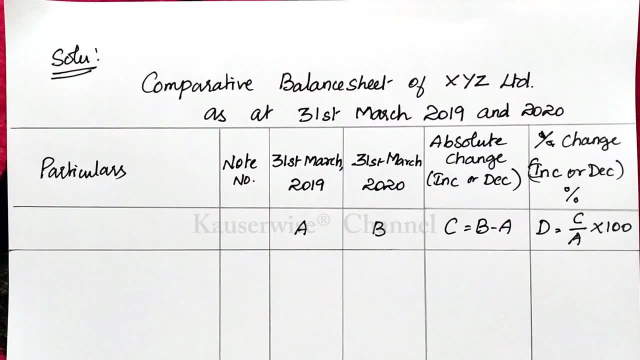 in the comparative statement of balance sheet. Okay, we are going to compare each and every component of balance sheet Okay, which pertaining to two different years. Now let us see the calculation part. So first we need to enter all the assets and liabilities which is given in the 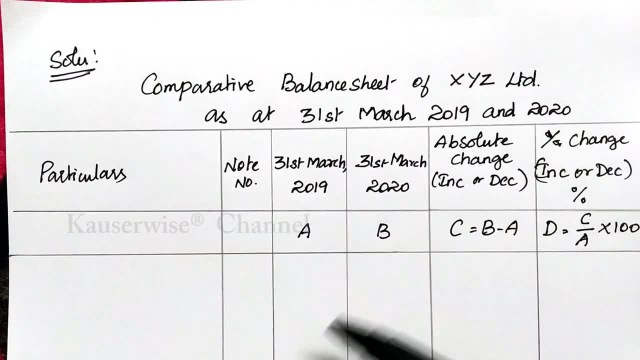 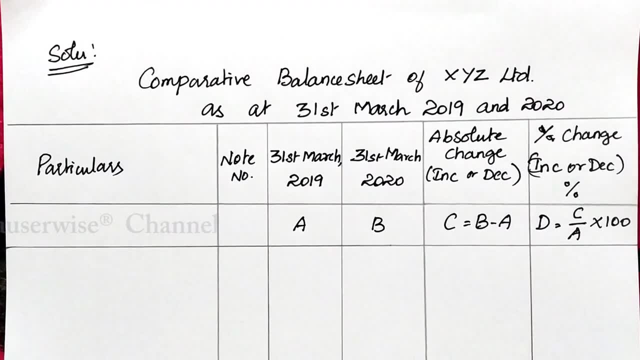 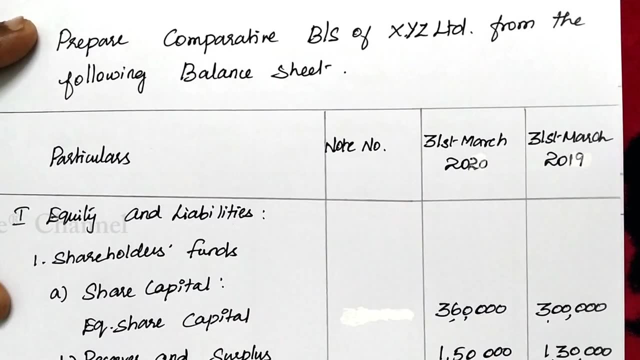 problem, and then we need to enter previous year information and current year information as per the data given in the problem. Then only we can go for the other two calculations. Let us see the first three things, That is, particular column, previous year data and current year data. First step is we need to enter all the 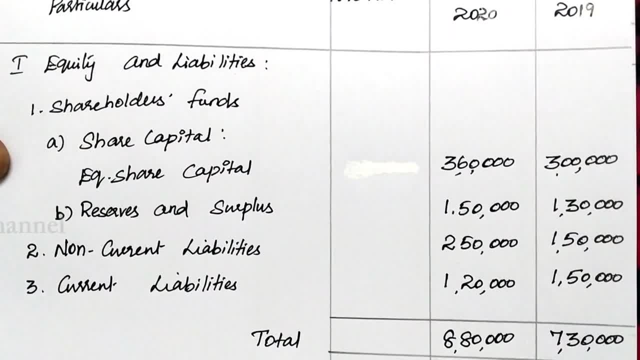 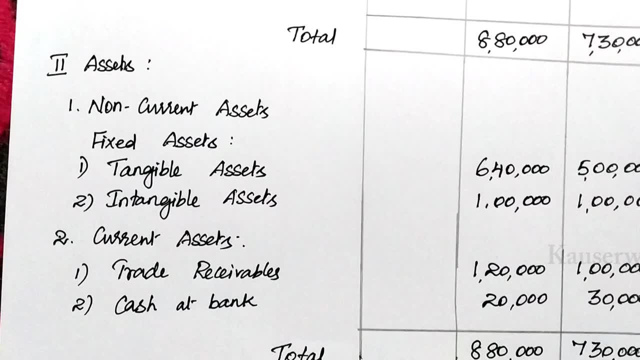 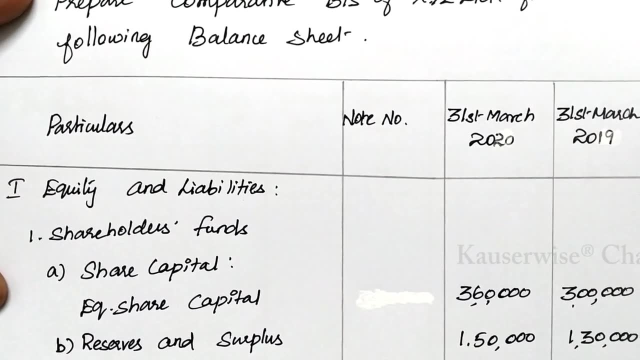 liabilities and asset, as per the problem. Okay, enter all these items in the solution in the first column, That is particular column, and the next one is in this problem. they have given data for the current year first and previous year next. Okay, but according to our calculation, first we 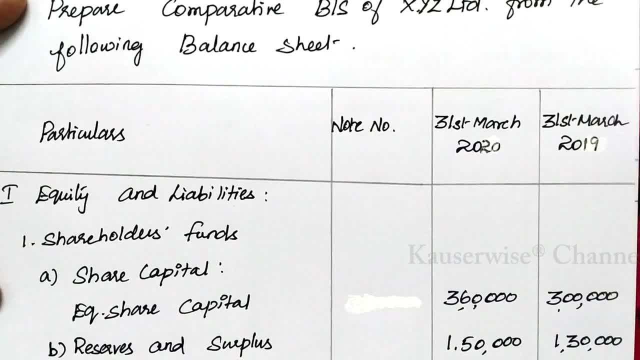 need to enter the liabilities and assets as per the problem. So we need to enter all the liabilities and assets as per the problem. So we need to enter all the liabilities and assets as per the problem. Now we can enter previous year information in the first column and in the next column we need to. 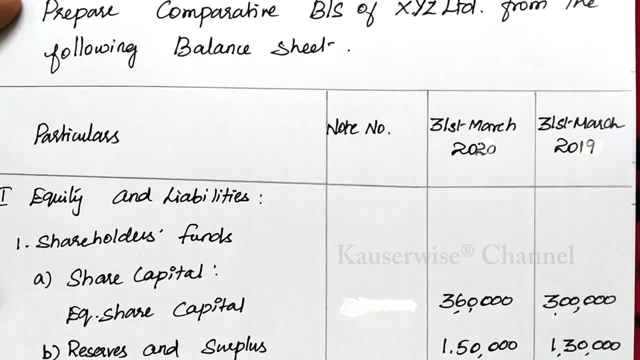 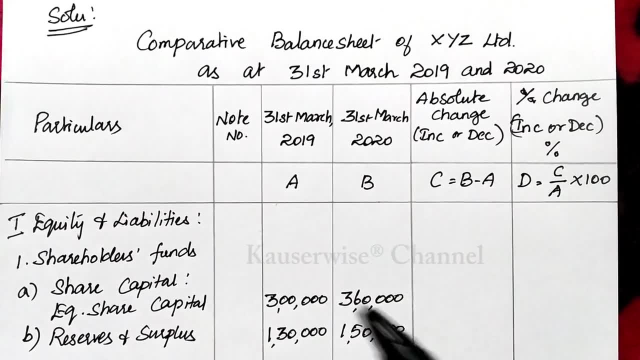 enter the current year information. Then only we can able to find out the difference. Then we can find out the percentage of change. Okay, let us see the solution. See the solution. we have entered all the liabilities and assets which is given in the problem and we have entered the values for. 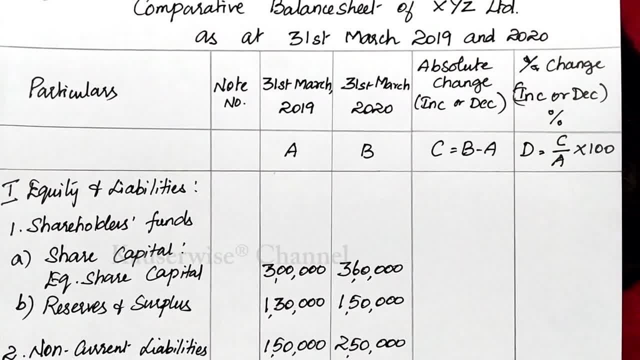 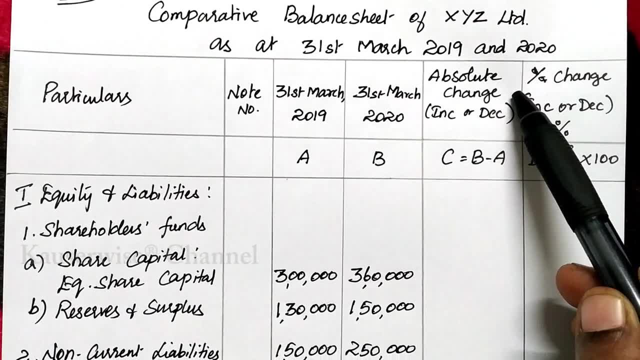 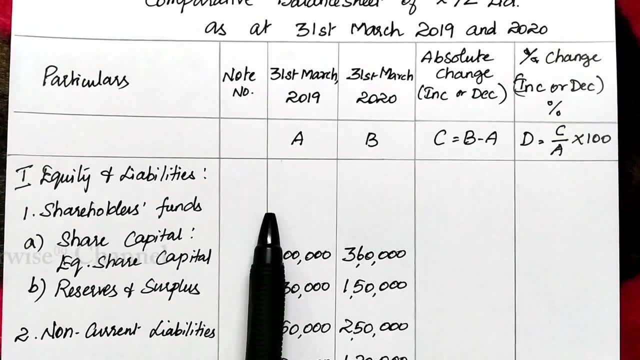 previous year and current year, as per the problem. Okay, now, after entering all these things, the next step is we need to find absolute change. that is, we need to find increase or decrease by comparing- okay, current year data with the previous year data. then we'll be getting c. c means absolute. 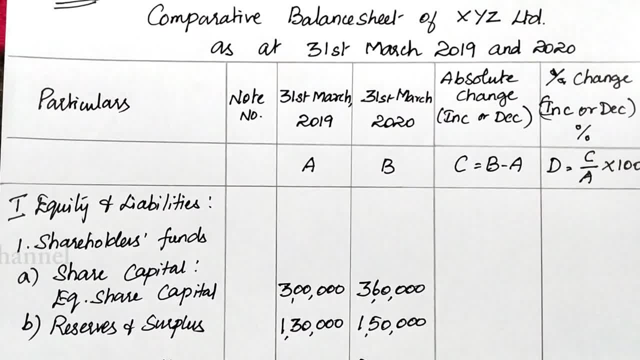 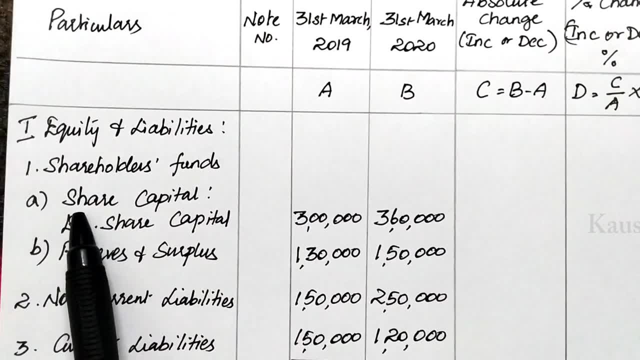 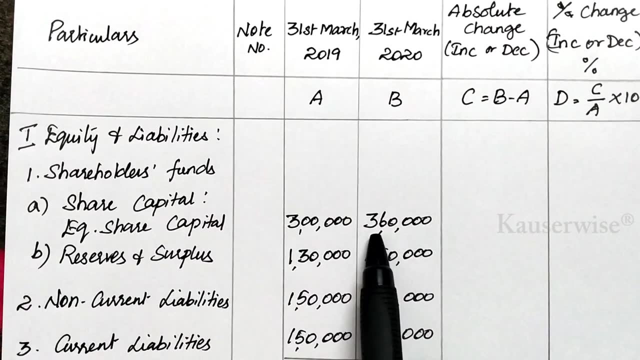 change. okay, now let us see the calculation of absolute change by comparing 2020 data with 2019 data. see the first one. that is a share capital, equity share capital. so current year: 360, previous year: 3 lakhs. the difference is 60 000 increased. okay, plus value in case of any negative value. 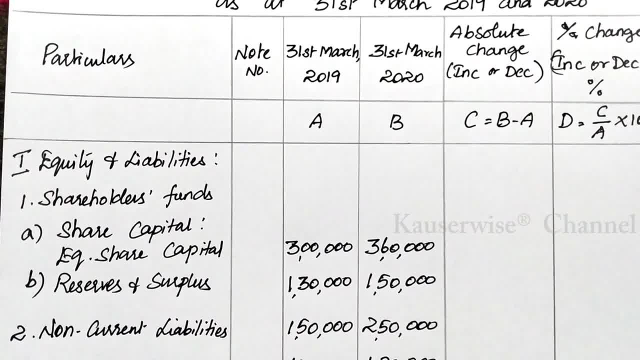 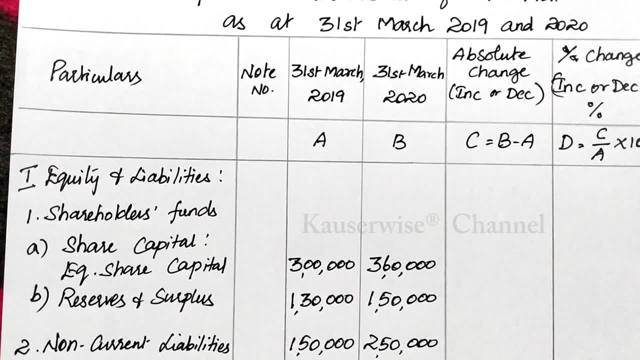 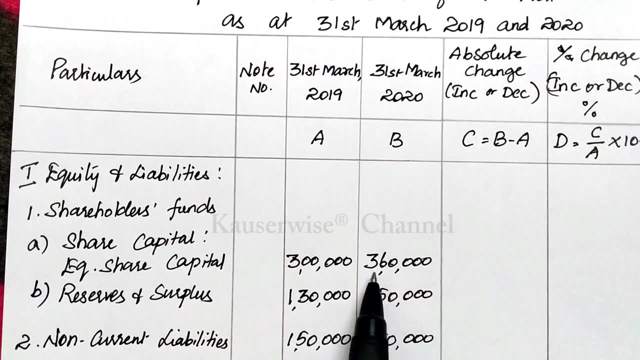 we need to enter the negative value within the bracket. okay, the same thing, even applicable for percentage. for negative value, we need to enter the value within the bracket, okay. see the first one: the current year equity share capital: 3 lakh 60 000. previous year: 3 lakhs. what is the difference? 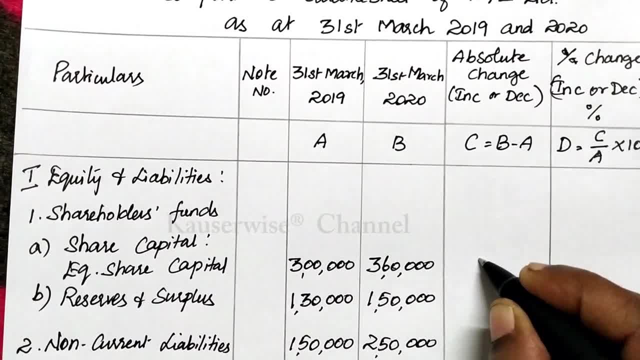 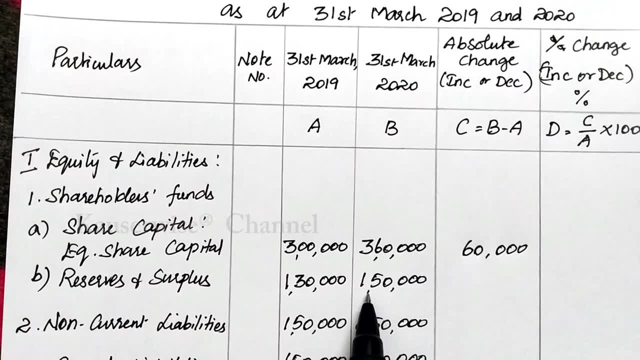 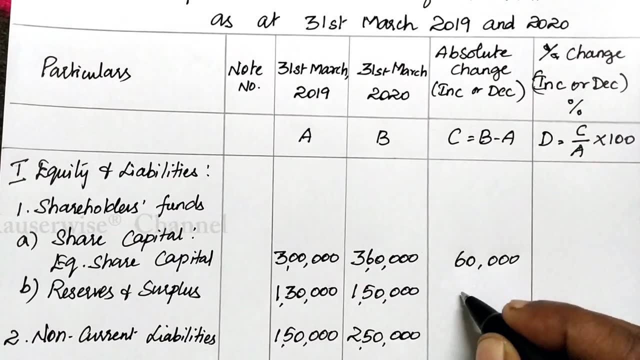 3 lakh 60 minus 3 lakhs: 60 000 increased. okay, so enter 60 000. the next one is a resource and surplus. current year, how much? 1 lakh 50. previous year, 1 lakh 30. so what is the difference? 20 000 increased current year, so enter here 20 000. the next one: 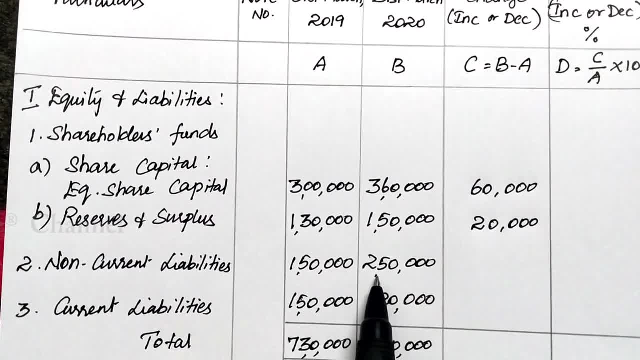 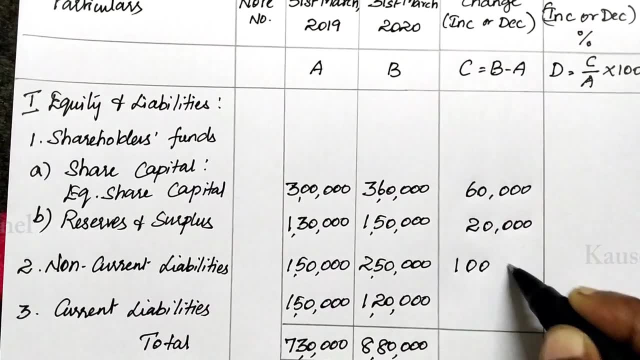 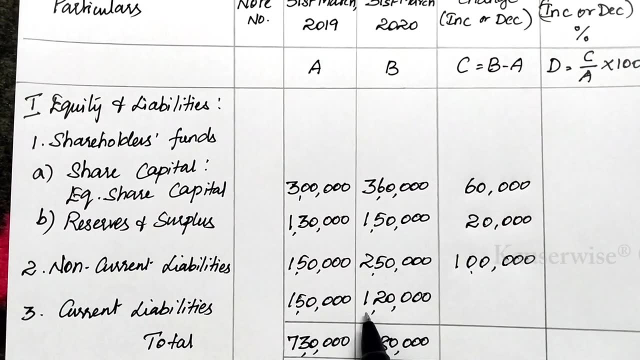 non-current liabilities: current year: 2 lakh 50 000. previous year: 1 lakh 50 000 difference: 1 lakh increased. so enter 1 lakh 60 000 plus 1 lakh 20 thousand. okay, so current year current liability is 1 lakh 20 000 previous. 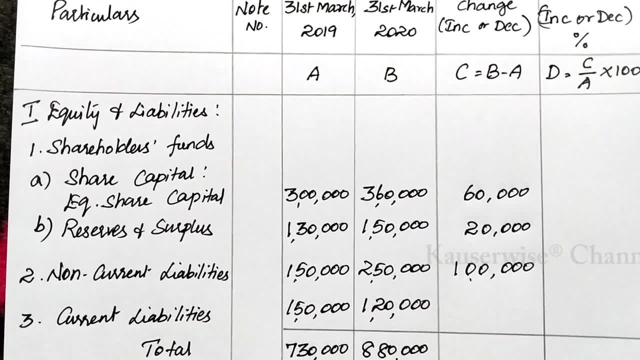 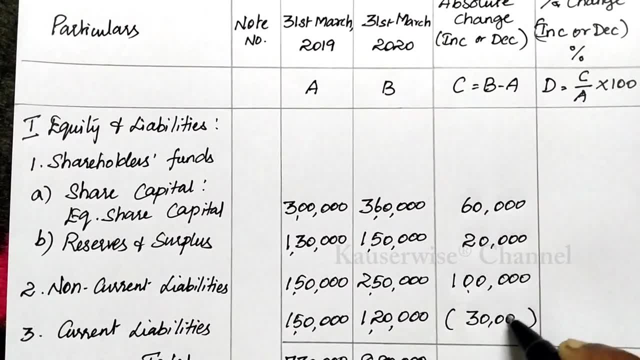 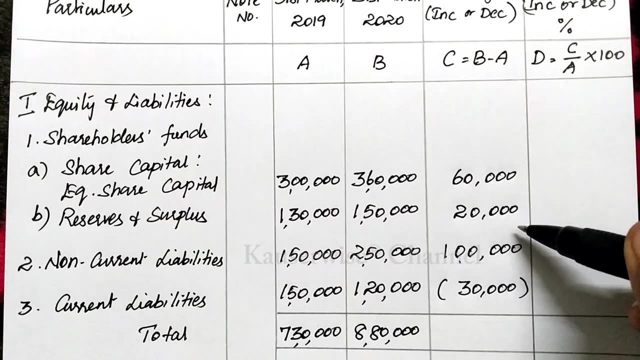 year 1 lakh 50 000. so difference how much? 30 000 decreased. okay, so we need to enter 30 000 within the bracket. okay, see, now we need to find out the total. okay, so total: 60 000 plus 20 000, 80, 80 plus. 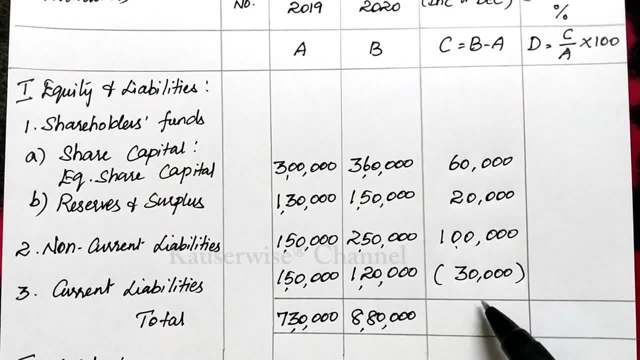 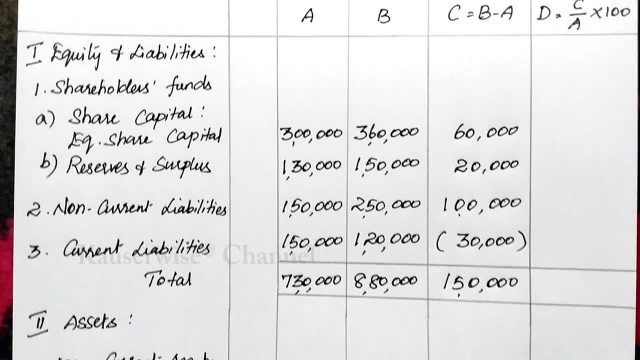 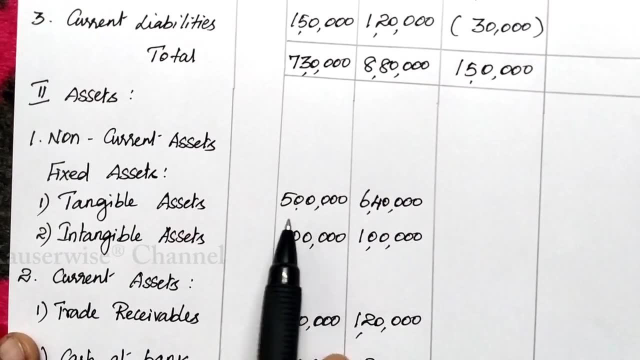 1 lakh. 1 lakh 80 000 minus 30 000, the answer will be 1 lakh 50 thousand. okay, enter 1 lakh 50 thousand here. in the same way, find out the absolute change for assets. also see current year tangible asset: 6 lakh 40. previous year: 5 lakh. how much increased? 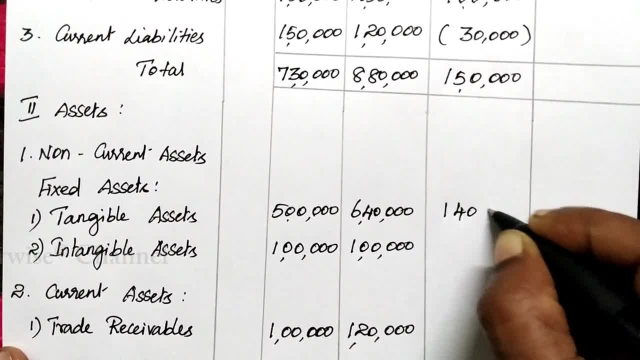 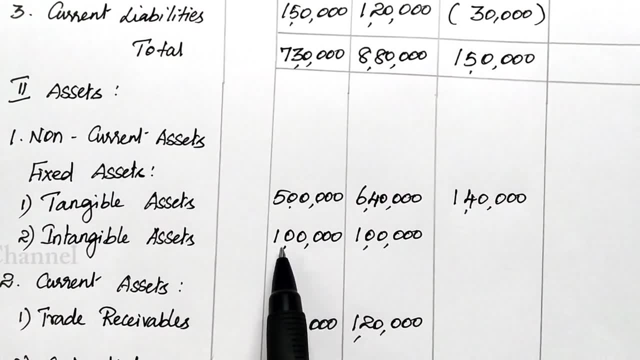 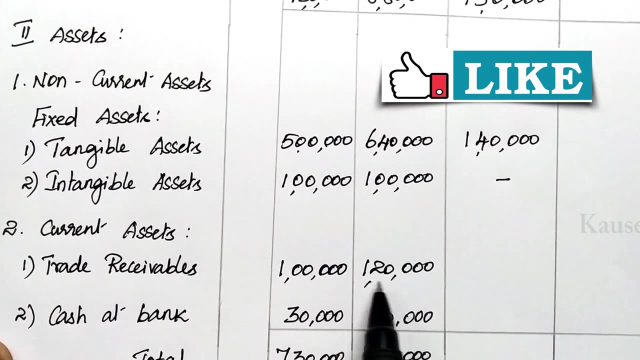 1 lakh 40 thousand increased. okay, so 1 lakh 40 thousand. the next one: tangible asset for tangible asset: current year: 1 lakh. previous year also 1 lakh. there is no changes, so put dash. the next one: trade receivables: current year: 1 lakh 20. previous year: 1 lakh. so what is the difference? 20 000. 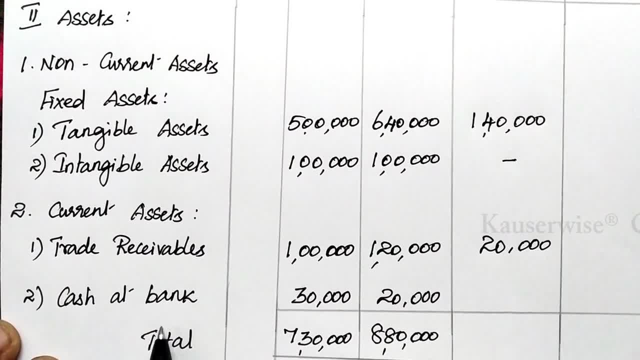 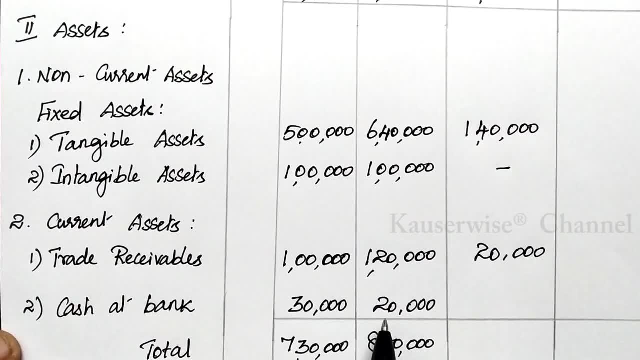 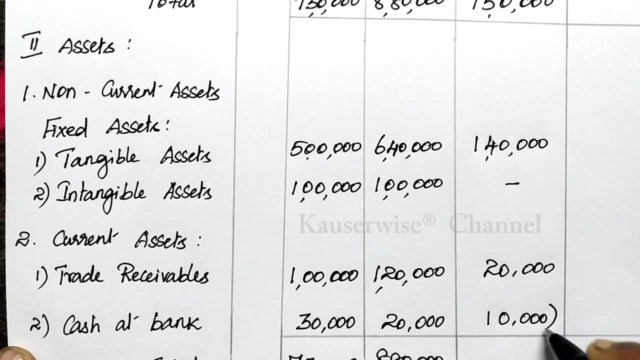 increased. okay, and the next one: cash at bank. current year 20 000. previous year: 30 000. the difference is 10 000 rupees decreased. okay, so current year value is lesser than the previous year value, so that minus 10 000. no, this will be entered within the bracket. okay, now find out the. 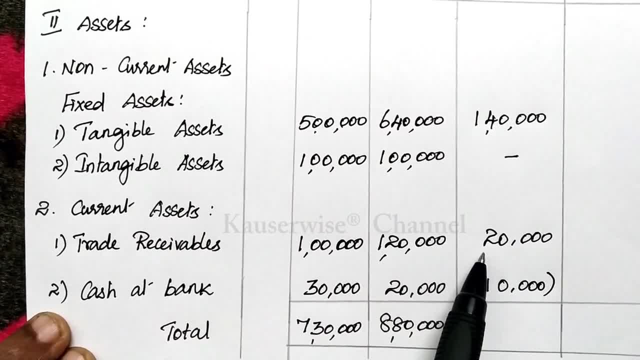 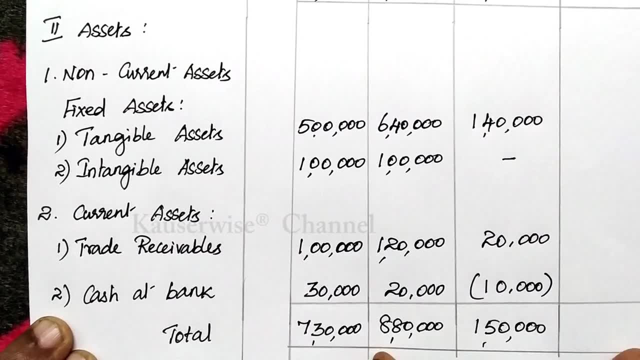 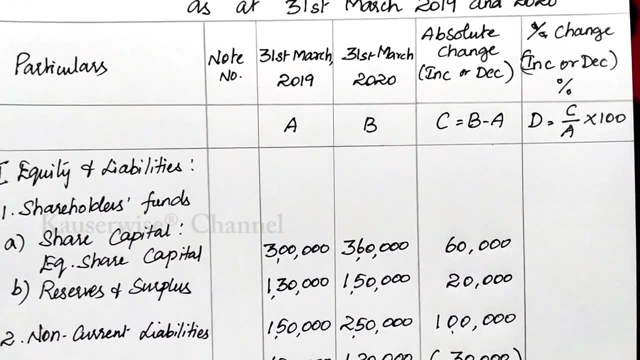 total, 1 lakh 40 plus 20, 1 lakh 60 minus 10 000, you will be getting 1 lakh 50 000. okay, so this is the way to calculate absolute change. it may be increase or decrease according to the data given in the problem. the final step is: 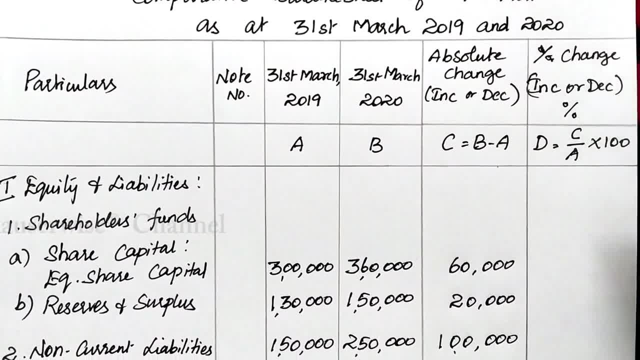 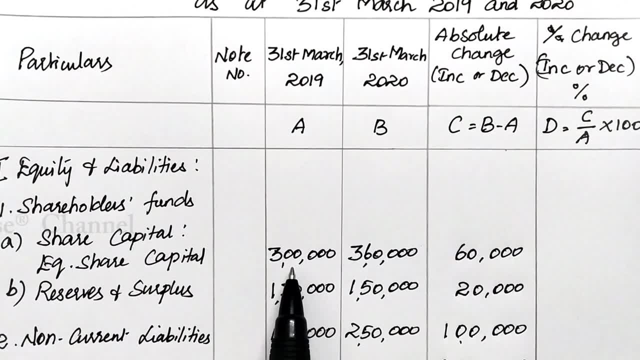 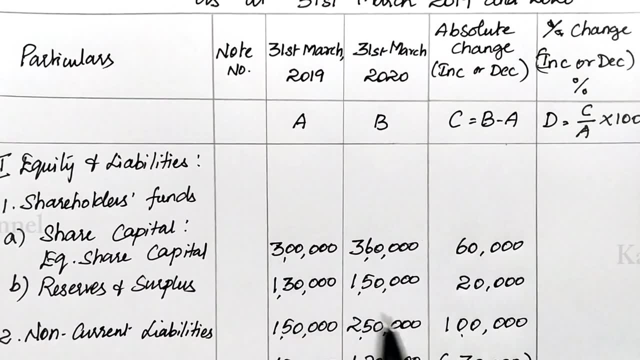 we need to find out the percentage of change by using the formula that is a change, absolute change divided by base year. base year is previous year is the base year. that is a okay. so 60 000 divided by 3 lakhs into 100. the same way, 20 000 divided by 1 lakh, 30 into 100, and then 1 lakh divided by 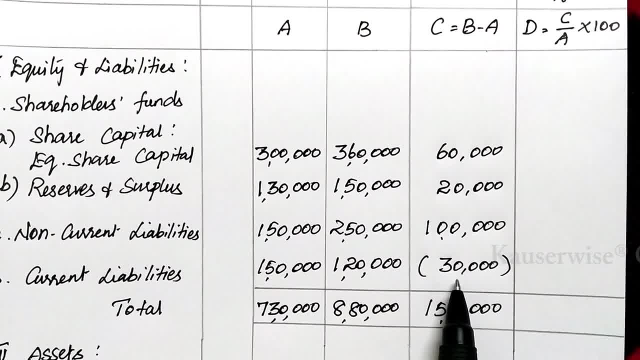 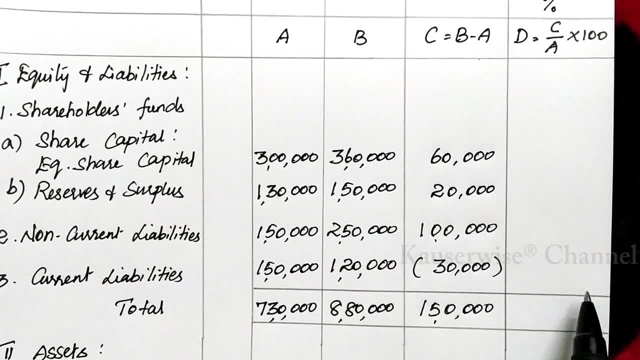 1 lakh 50 into 100 and the next one minus 30 000 divided by 1 lakh 50 into 100, you will be getting negative percentage. okay, that will be entered within the bracket. in the same way, we need to find out the percentage of change. okay, so this is the way to calculate absolute change. 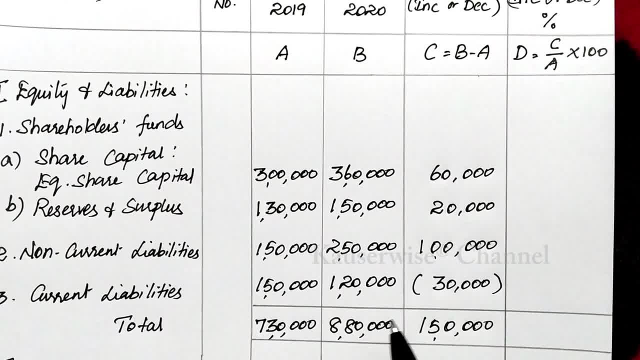 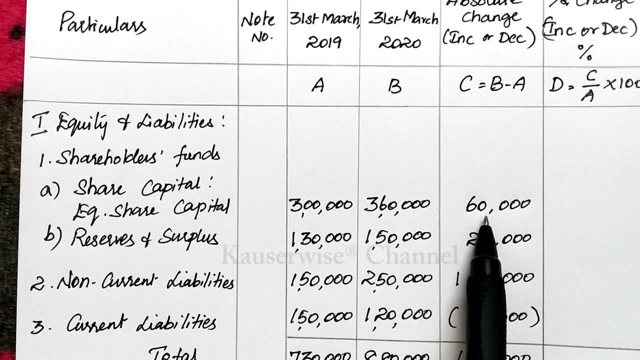 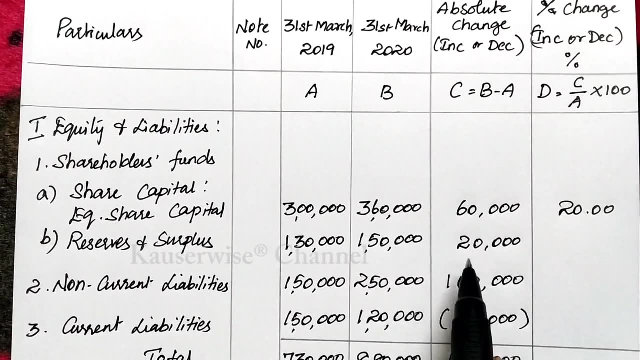 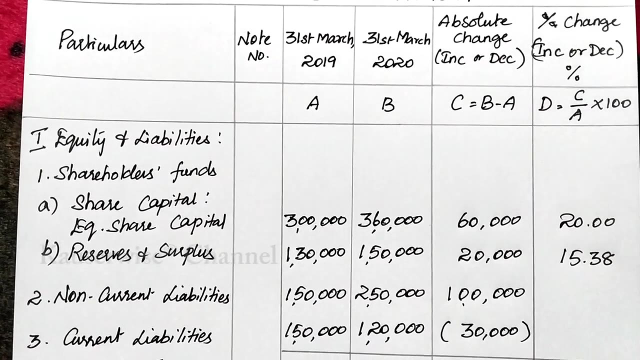 percentage change for each and every components of assets, as well as liabilities. now see the calculation of percentage change. the first one: 60 000 divided by 3 lakhs, into 100- 20 percentage. and the next one: 20 000 divided by 1 lakh, 30, into 100- 15.38. okay, the next one: 1 lakh divided by 1. 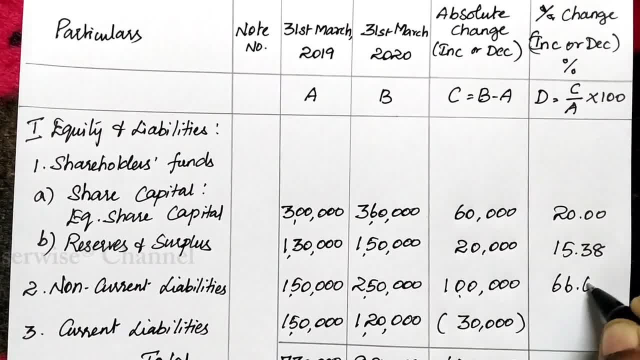 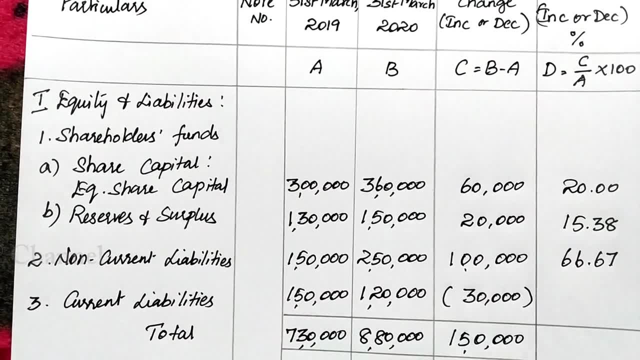 lakh 50 into 100. 60 000 divided by 1 lakh 50 into 100. 60 000 divided by 1 lakh 50 into 100: 66.67. okay, and the next one minus no. so minus 30 000 divided by 1 lakh 50 into 100, you will be. 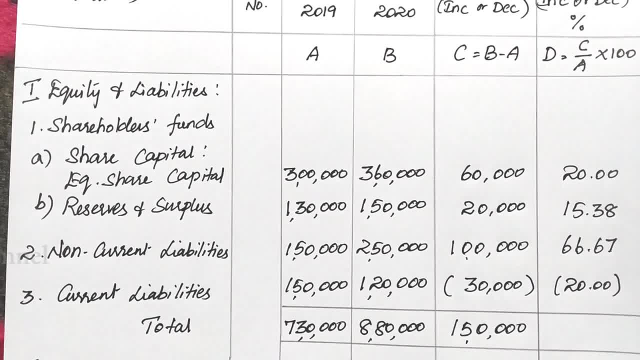 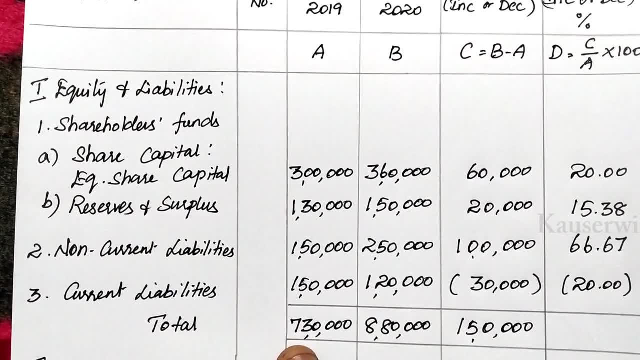 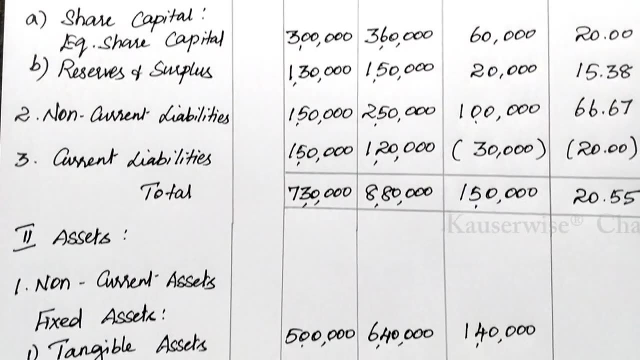 getting minus 20 percentage. okay. now we need to find out the percentage change, even for total. okay, 1 lakh 50 000 divided by 7. lakh 30 into 100, you will be getting 20.55 percentage. okay. the next one assets, the first one: 1 lakh 40 divided by 5. 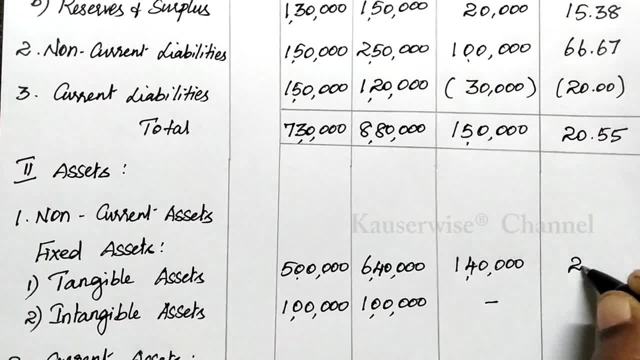 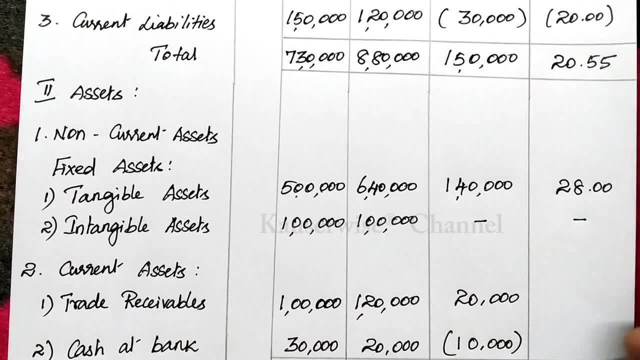 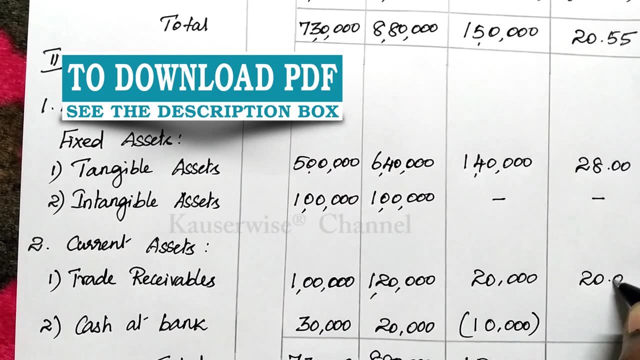 lakhs into 100, you will be getting 28 percentage. the next one 1 lakh. 1 lakh. there is no change. no, so put dash, even for percentage, and the next one: 20 000 divided by 1 lakh into 100, you will be getting 20 percentage and the last one minus no. 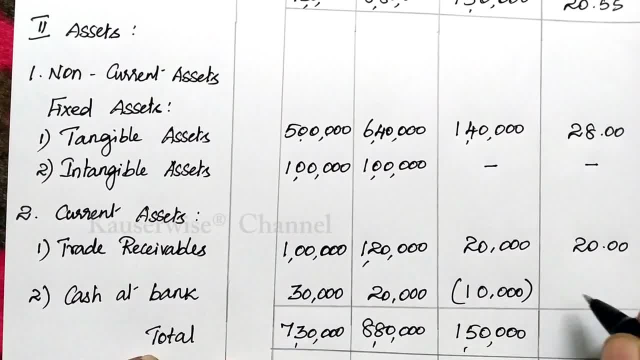 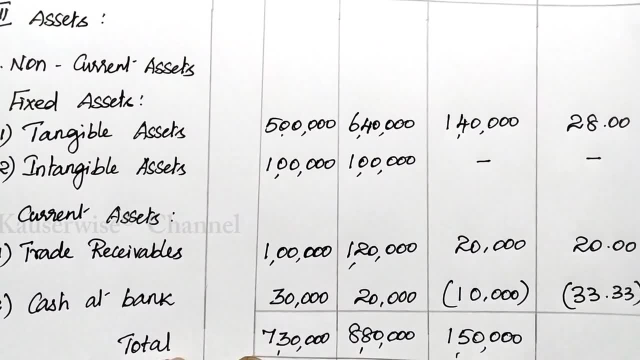 so minus 10 000 divided by 30 000 into 100, you will be getting minus 33.33 percentage for minus. we need to enter within the bracket. in the same way, we need to find out the percentage change in. we need to enter within the bracket. okay, the last one. we need to find the percentage, even for total.